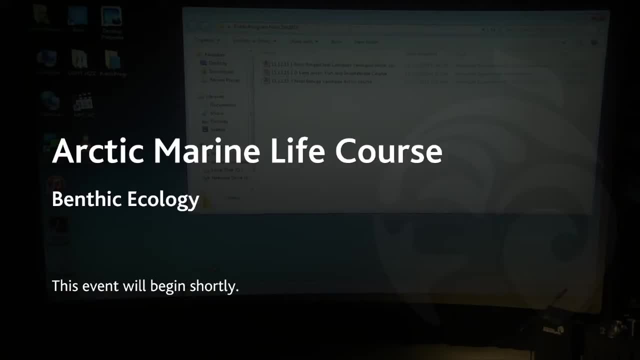 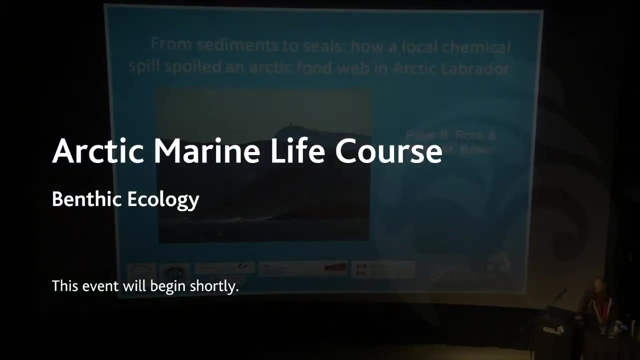 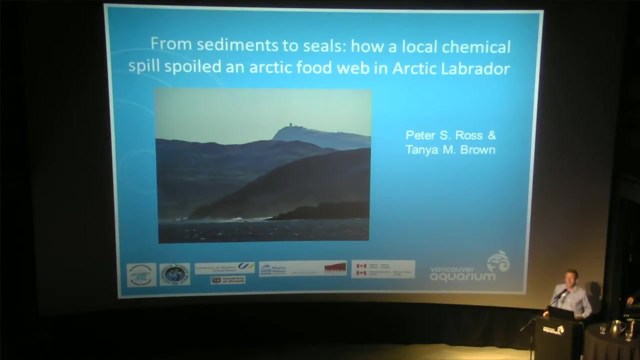 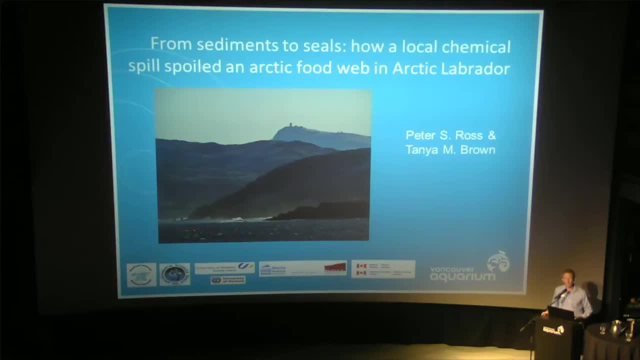 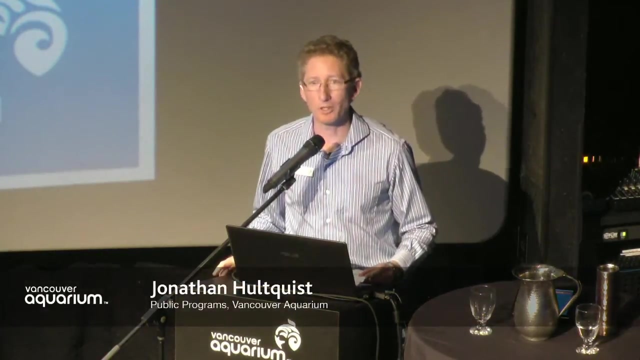 How do people living in the southern parts of Canada, or anywhere else in the world for that matter, learn about this unique and fascinating marine? learn about the unique and fascinating marine animals that inhabit this enigmatic environment. Let me present to you the online Arctic marine life course. 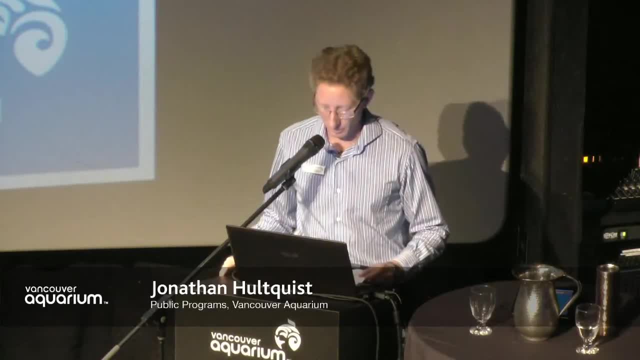 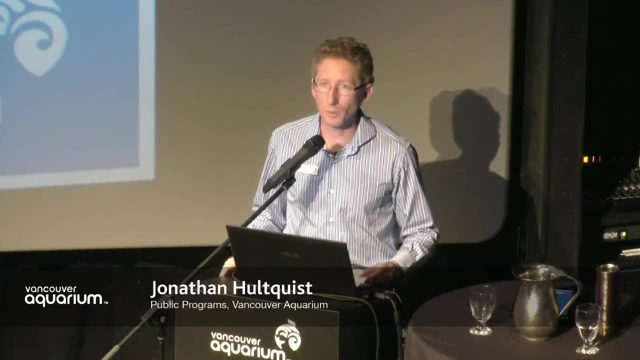 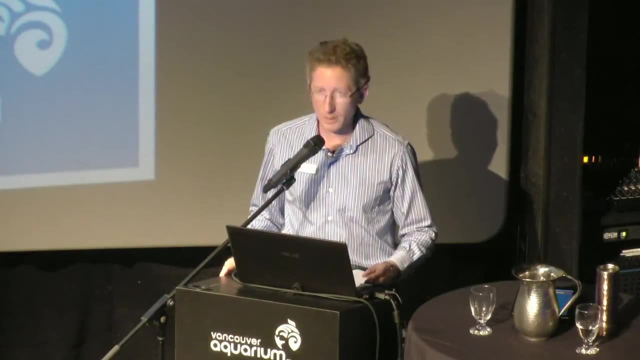 The course is supported by the Science in Canada's North Cafe Scientifique series and we would like to acknowledge the support of the W Garfield Weston Foundation and the Canadian Association of Science Centres for their support. Our partners include the Alliance of Natural History Museums of Canada, Canada's accredited zoos and aquariums. 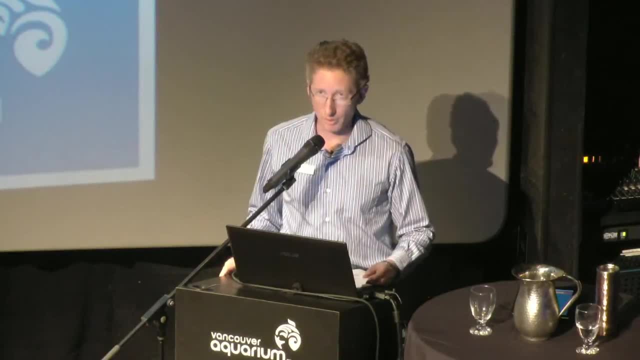 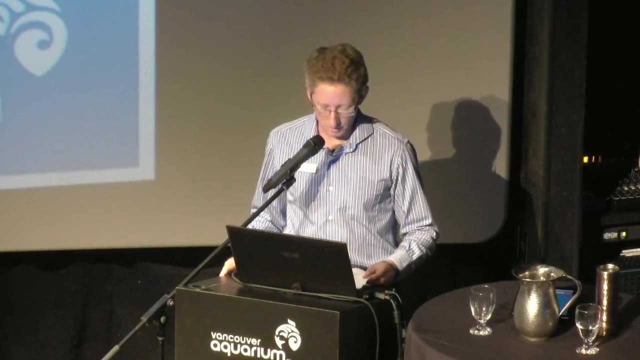 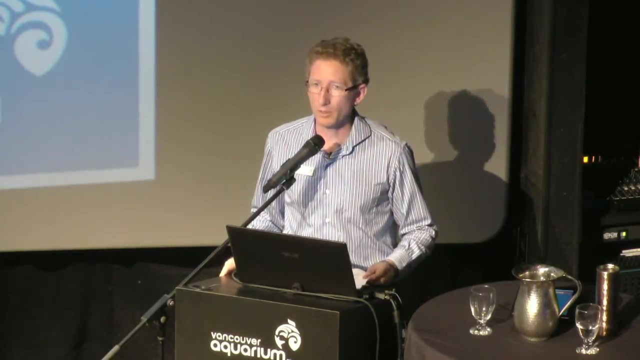 TELUS SPARC in Calgary, the Canadian Museum of Nature in Ottawa and the Discovery Centre in Halifax. Keep track of the dates and locations of all of our presentations on our website, wwwvanaquaorg slash- Arctic Marine Life course. 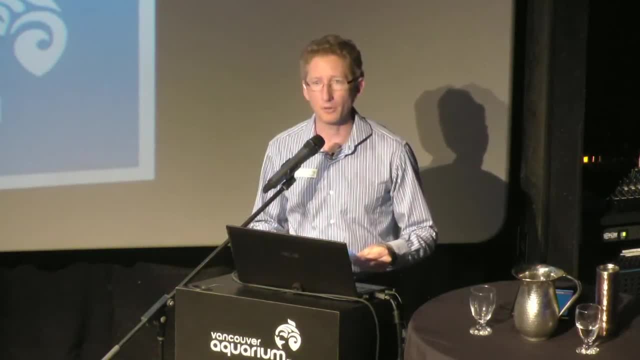 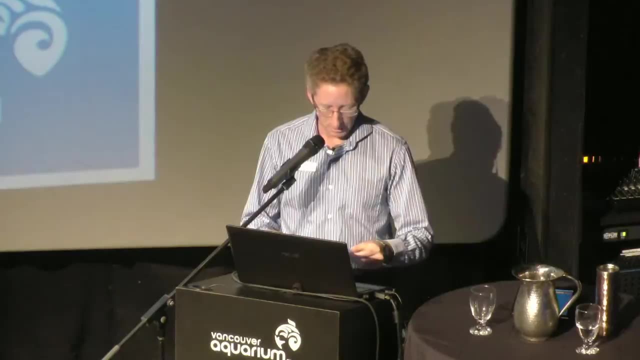 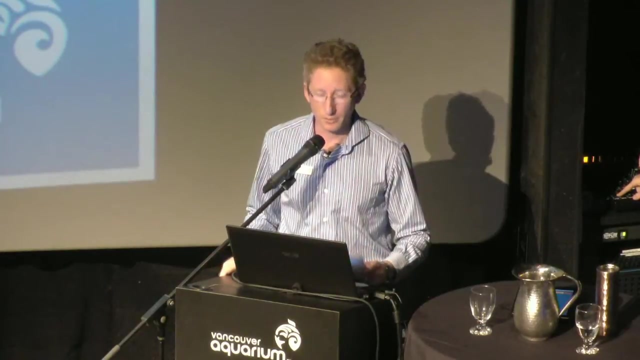 If you miss a presentation, you can always watch it online after it's been recorded. If you have any questions about the course or you would like to register, you can contact me at jonathanholtquist at vanaquaorg. Our speaker is Dr Peter Ross. 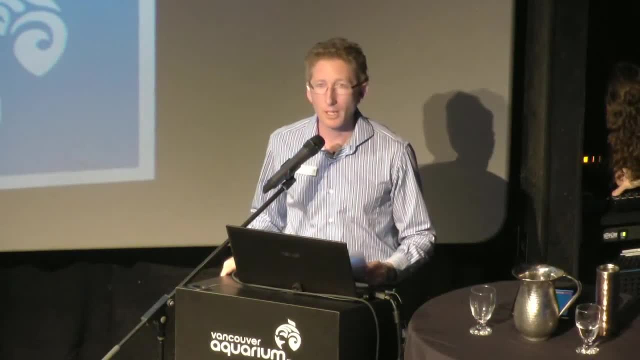 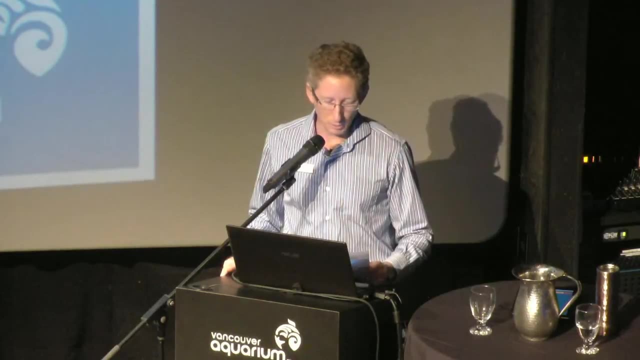 Director of the Ocean Pollution Research Program at the Vancouver Aquarium Marine Science Centre. Peter's research focuses on evaluating the effects of pollutants on the health of marine animals. He has collaborated on a number of studies conducted in the Arctic. His presentation will focus on benthic ecology and how pollutants can be used to map food webs. 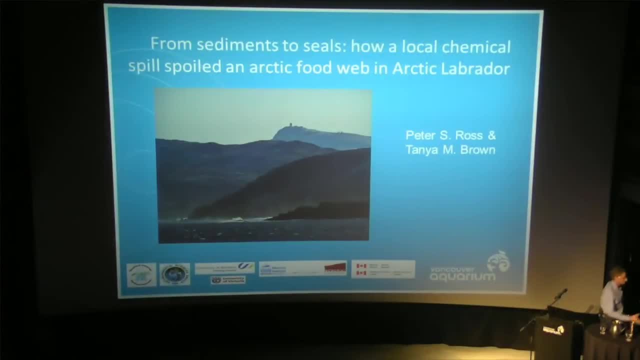 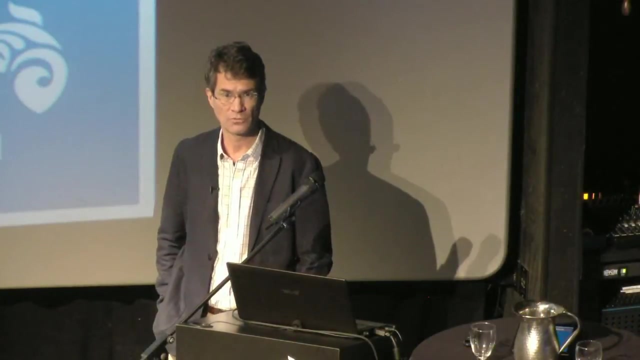 Dr Peter Ross. Thank you and welcome everyone to this evening's lecture. I'm delighted to be here. I am not a benthic ecologist, but I can tell you that benthic ecology is the foundation for much of what I do when I look at ocean pollutants. 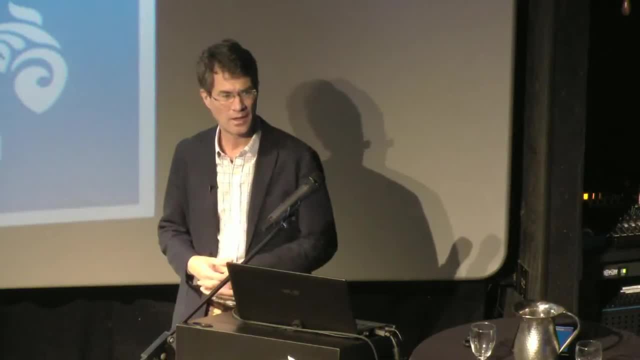 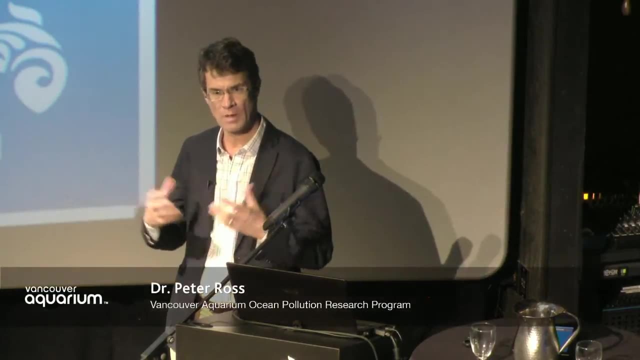 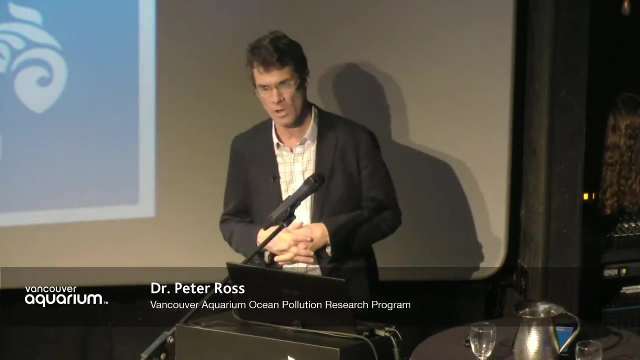 So what I'm going to do tonight is explore the sediments and the sea bottom and provide a little bit of a segue into the invertebrates and into the fishes and the birds and the mammals that we're looking at, And to do this I'm going to take you 8,000 kilometres to the east of Vancouver and a little bit north up into Arctic Labrador. 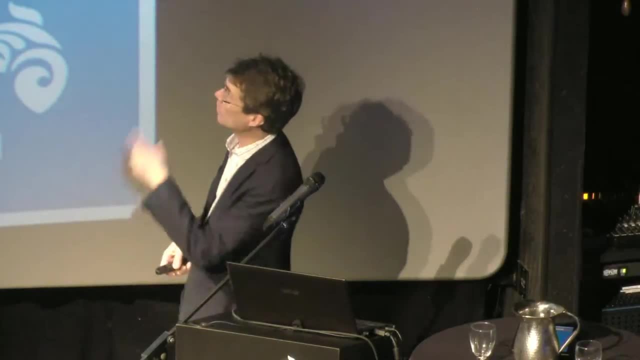 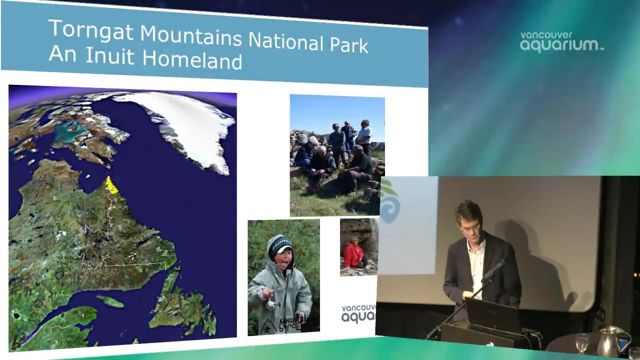 That will be the focus of this talk tonight. I'd like to acknowledge my co-author, Tanya Brown, who spent much time in this location- much more time than I did- And let me start by saying this is a very special place. It's a spectacular place that very few Canadians have visited. 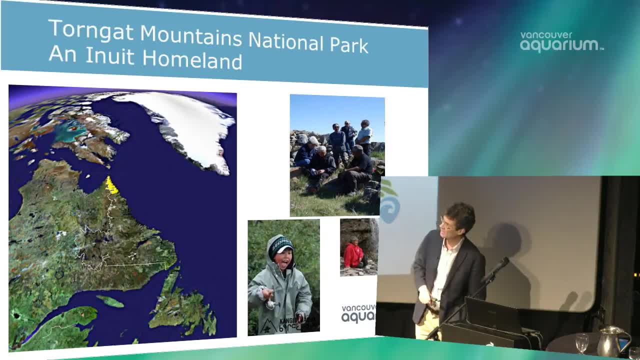 This is northern Labrador. If we look at that little yellow shaded region in this slide on the left, you'll see the Torngat Mountains National Park. This is a gem of a spot at the northern tip of Labrador and it's been used for millennia by Inuit. 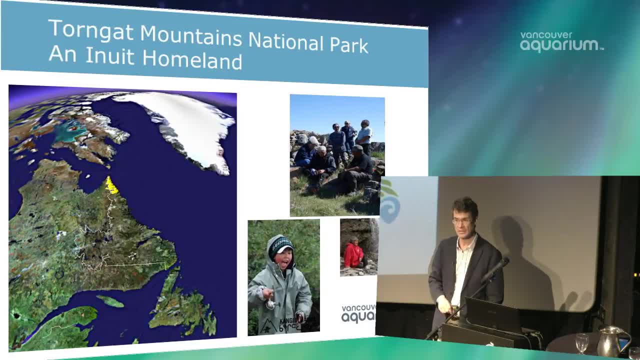 people who have relied on that interface of land and sea. You'll also note that this is not only an Arctic region. This is at the confluence of the Northwest Atlantic Ocean and the Arctic waters of Canada and the archipelago that we know of as the Canadian Arctic. 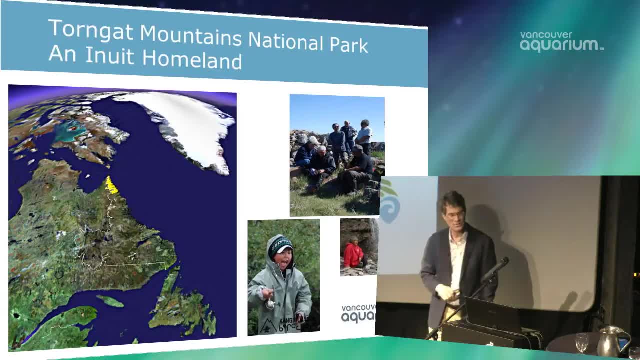 So this area just to the east of here were also was also the site where the Franklin Expedition traversed in the late 1840s as they sought the Northwest Passage, and disappeared until the well, until we discovered a little bit more about what went wrong with their journey and their expedition. 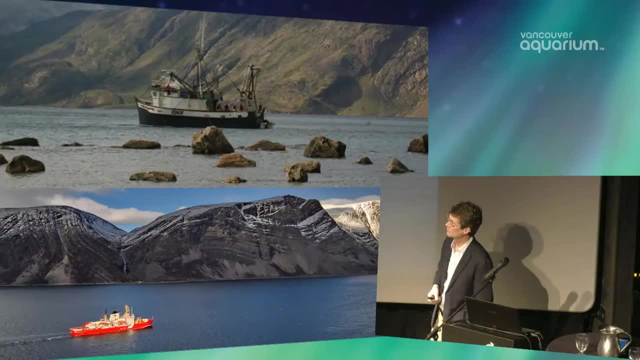 So spectacular spot, a spot that few get to and a few people get to this part of the world because it's it's really tough getting there. It'll take you two days by air to travel, Or if you're doing fieldwork there, you'll be fortunate. 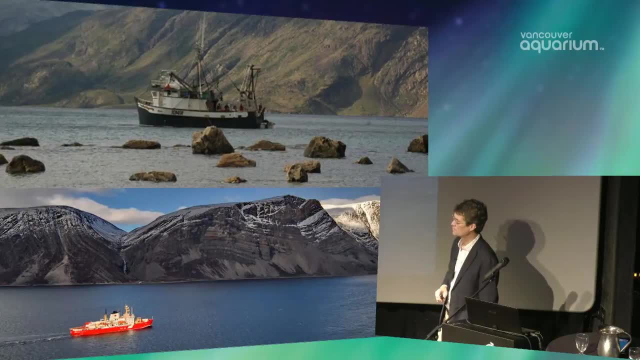 if you can get aboard one of the Canadian Coast Guard icebreakers that that transit these waters- coastal waters heading into the eastern Canadian Arctic or, more appropriately, when you're dealing with nearshore environments in some of the coastal waters in these areas, Working with some of the Inuit fishermen that know the waters very, very well. 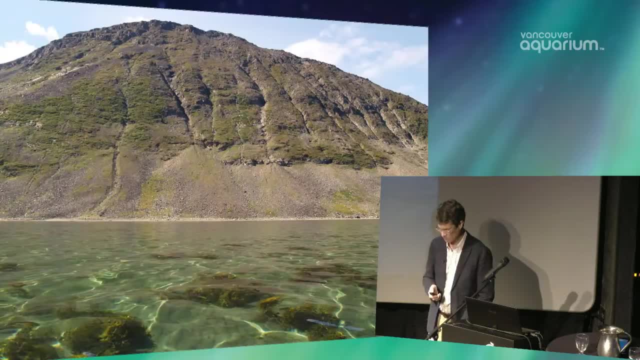 know the elements and know the creatures that move about these waters. And when we look at this topography, we, as humans, we look at the, the land. That's what we understand. We are air breathing, air breathing animals. We stand on a shoreline. 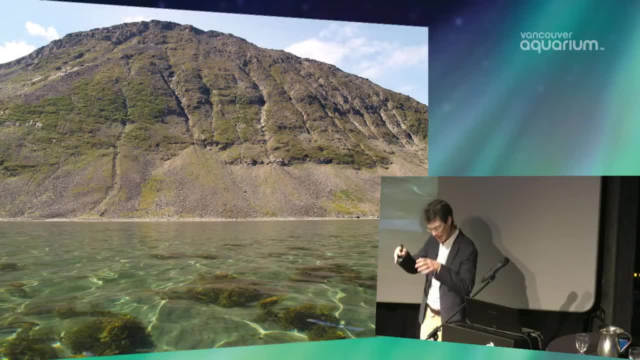 We look out to sea, We see the surface of that sea and what lies below the surface that those waters represents a bit of a mystery To most of us, And it's that interface that I would like to talk to you about today. We're going to go into the waters of a, a specific fjord in Labrador. 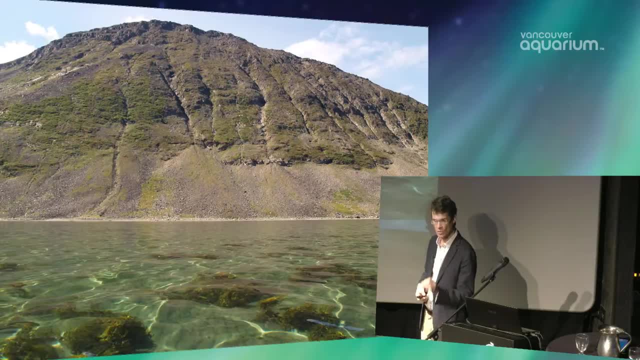 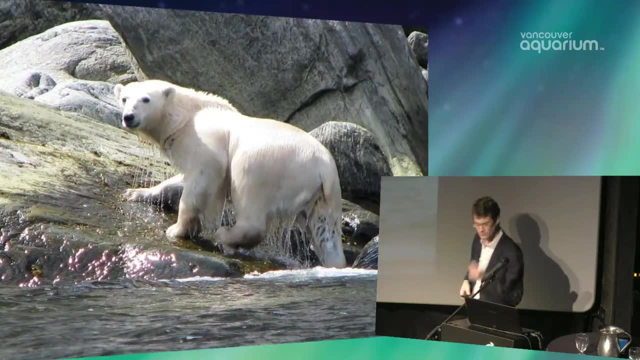 and try to understand a little bit more about why science or why Canadians might be interested in this part of the world and interested in benthic ecology, for example. This is a creature I'm not going to talk about tonight, but I thought I'd put this animal up there because what Arctic talk would be complete. 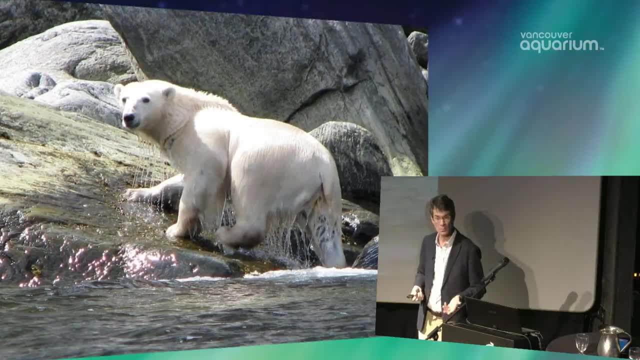 without a polar bear. Of course, these creatures are marine mammals. They do rely very heavily on marine mammals and fish for their subsistence and they can swim, swim around these coastal waters with impunity. So not the focus of this talk, but certainly a charismatic creature that does tell us a lot about the health of our oceans. 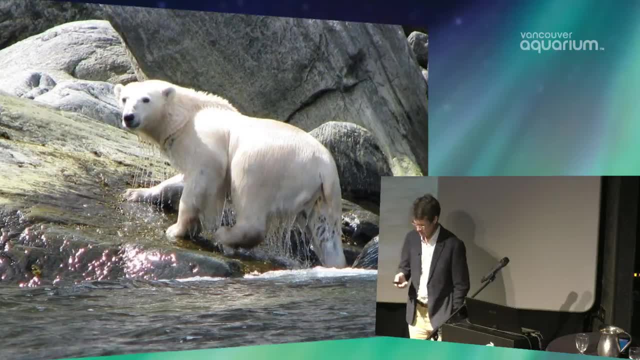 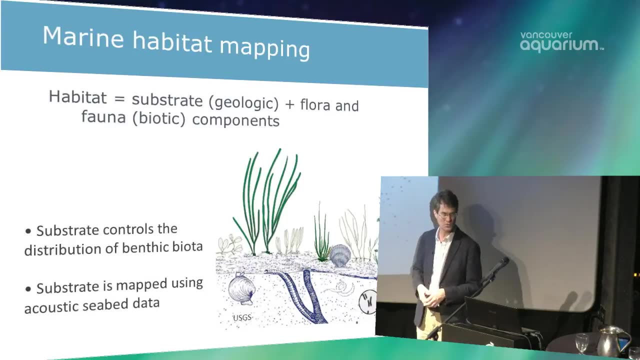 climate change, global pollutants and the food web, which I'll be talking about a little bit more tonight. And when we go down into the waters, we immerse ourselves subsurface and we go all the way down to the bottom of the sea. 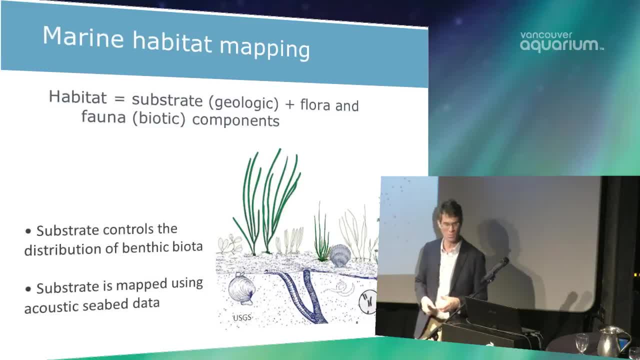 What do we run into? We run into substrate, We run into the sea bottom and there are various ways of studying that. We can do that with remote technologies. We can study it by dropping in sediment crabs. We can, as you'll hear shortly- 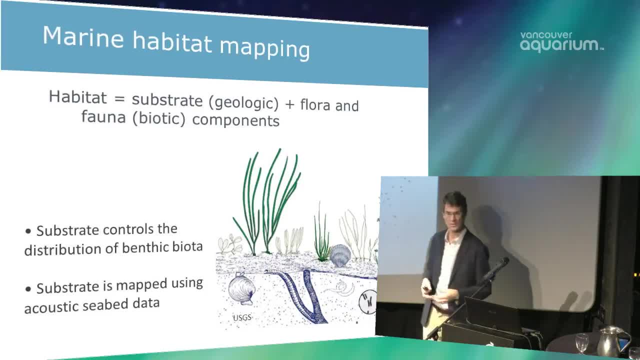 we can dive down with scuba gear and we can have a look at that substrate. That substrate can be one of a number of different things. It could be soft, It could be hard And it's sort of we're talking about something that is geologically. 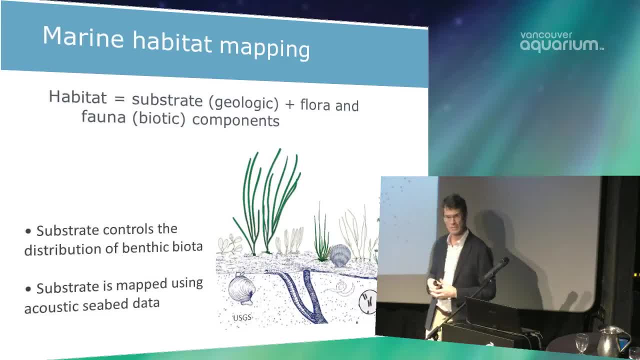 and geographically defined Ocean currents shape the way in which the substrate is formed and how it is characterized, And it's this substrate that forms the home for all the creatures that you and I would appreciate and understand and upon which much of our fisheries resources are dependent. 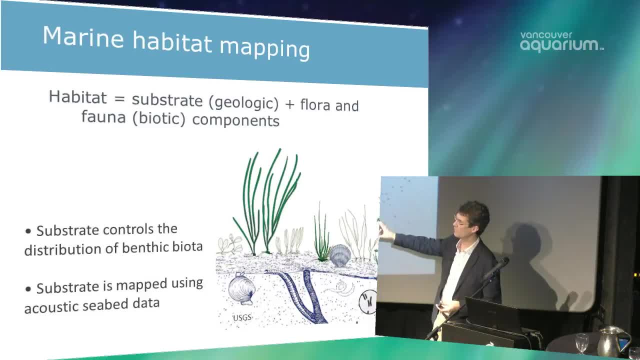 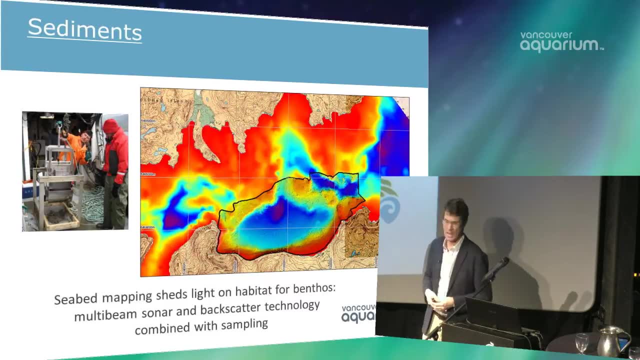 So this becomes habitat, geological, geographic and ultimately into the biological communities that you're hearing about tonight When we use seabed mapping. multi-beam sonar is one very powerful tool that is used extensively these days. That's simply being able to ping from a ship an array of sonar waves. 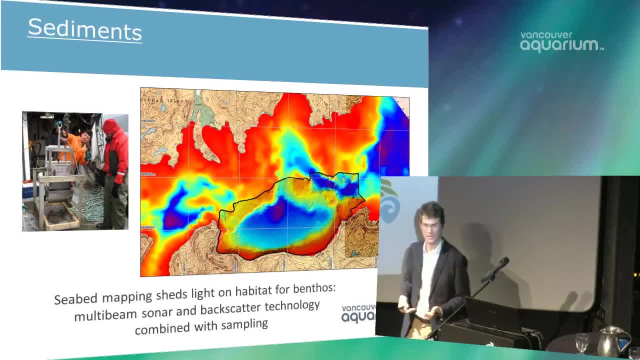 and getting a response, A response back at the ship which is then detected, And it's the time that it takes for that radar wave to hit the bottom and then bounce back up the ship that tells us how deep the water is, And it's the intensity of that signal that tells us something about the nature. 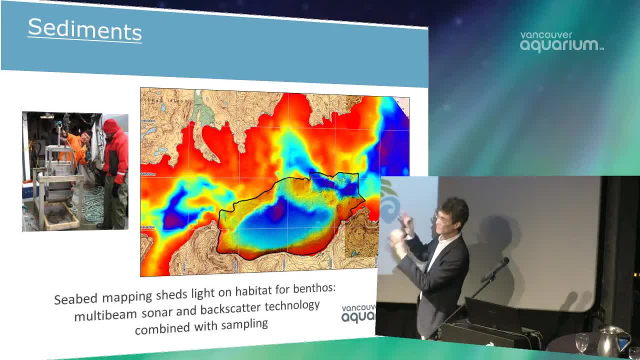 of the substrate, whether it's soft or whether it's hard, And we can start to create these wonderful maps that tell us about the substrate And if we know about the substrate and we start to unravel or uncover the relationship between that substrate and the sea life upon which that they reside and prosper. 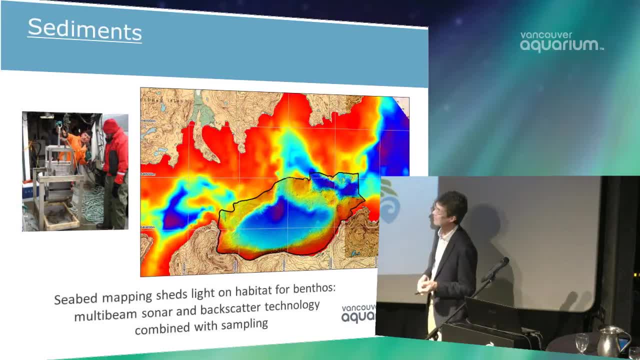 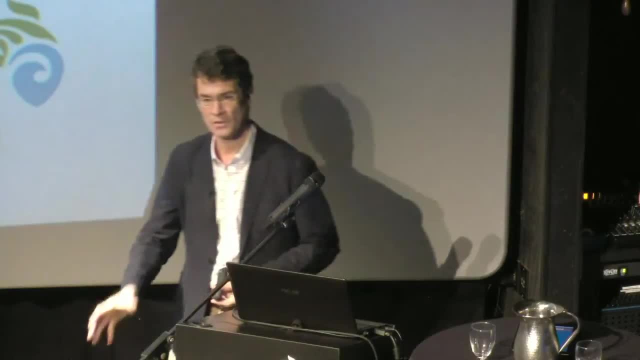 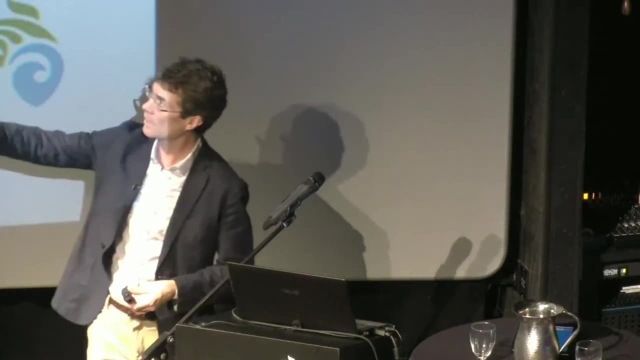 then we start understanding a little bit about home of those species. So in this picture here, the colorful one- the blue, represents deep water basins that are often filled in with light sediments because of ocean currents and natural sedimentation. You'll see the lighter colors and the red much shallower. 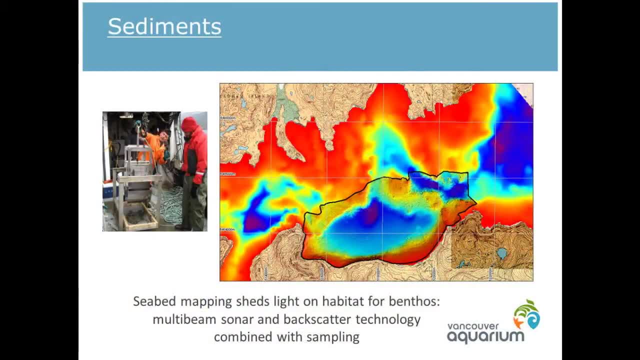 more scoured, more exposed to ocean currents, probably harder and more rocky and cobbly than the deep water basins, And you'll see a little bit more about that tonight. but it's something you can follow up later, Of course, when we get this technological glimpse at the bottom of the ocean. 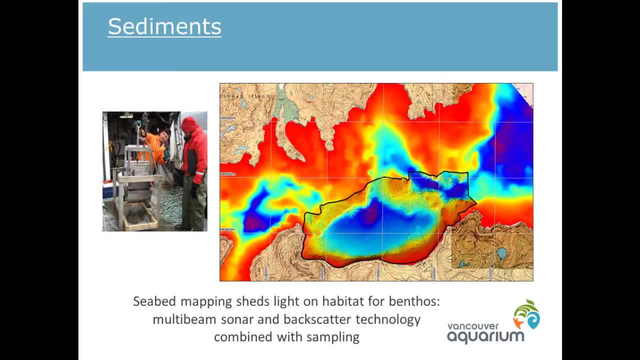 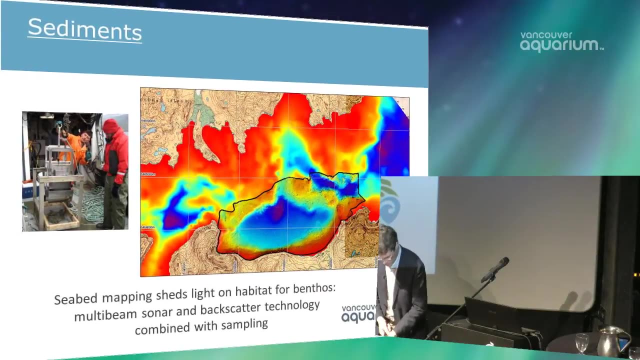 we want to ground truth, that We want to make sure we understand what that technology is in fact telling us. And on the left is a sediment sampling device called the Smith-McIntyre And that's something you drop on a line off the back of a vessel into the sediments. 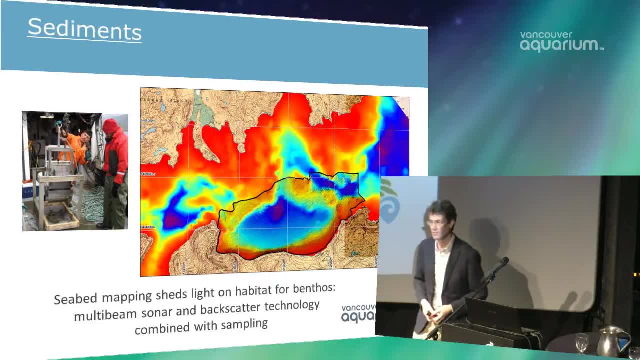 And it's like a shovel and it will grab the sediments and then you'll hoist them aboard the vessel. have a look at those sediments and you'll be able to see very quickly whether it's soft, cobbly, hard. 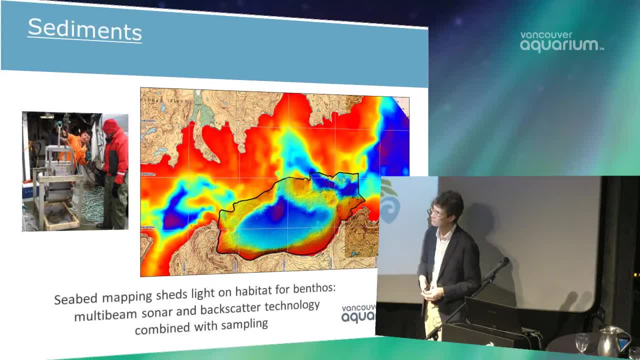 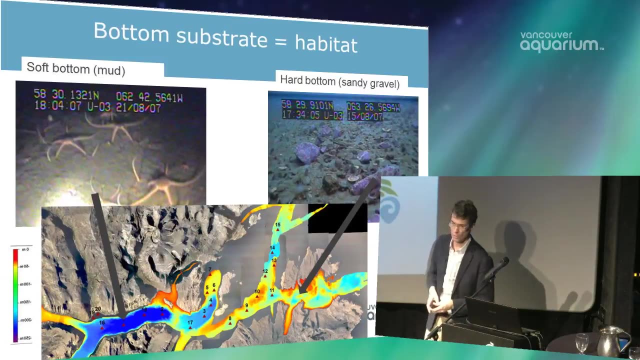 and you'll also get some samples of invertebrates in those samples. So, using a combination of different tools, we can understand a lot about the sea bottom, the sea floor, Which is habitat for a lot of different species, And in this case, if you send video down, you can have a look at the sea floor. 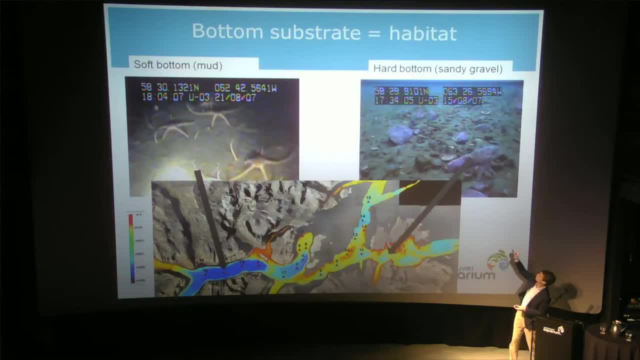 On the left you've got a soft bottom and you've got some brittle sea stars. On the right you've got a hard bottom surface, with all of the other species being associated with those, And that's when you can start to combine the multi-beam technology. 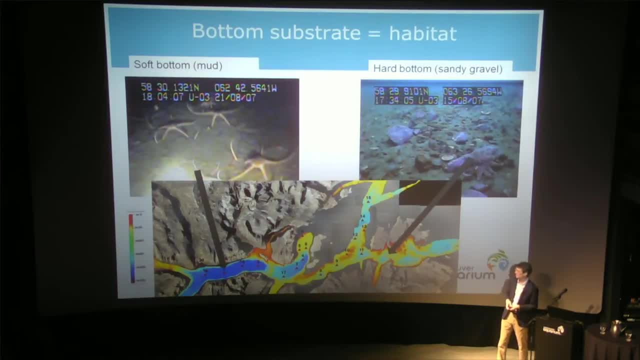 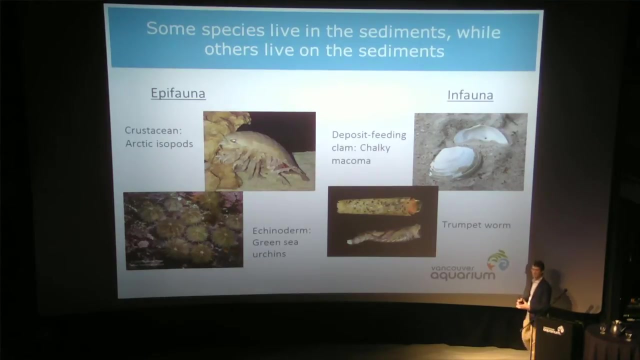 with another backscatter signal coming out of the multi-beam and get these habitat-based maps. What species are likely to be found In these different types of sea bottom or sea beds? And if we look at sediments, let's get a little bit away from the hard bottom for a minute. 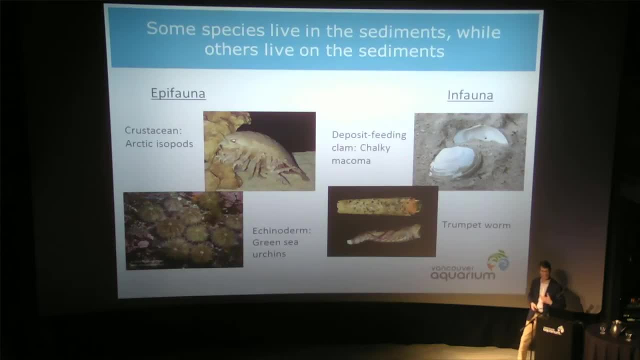 and just think about sediments. we can think about the creatures that live on the sediments versus the ones that live in the sediments, And we have both. There is a sediment food chain that thrives, and if you take samples of sediments, you'll see that. 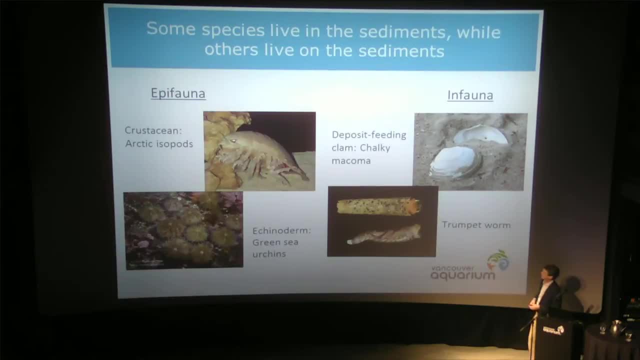 So we've got epifauna that will live on top of, on top of the sediments you've got in fauna. They'll be either inside the sediments or just at the sediment water interface. So some of the bivalves and clams you'll find buried in the sediments. 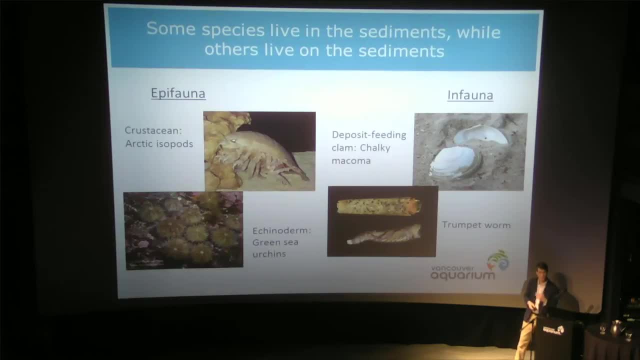 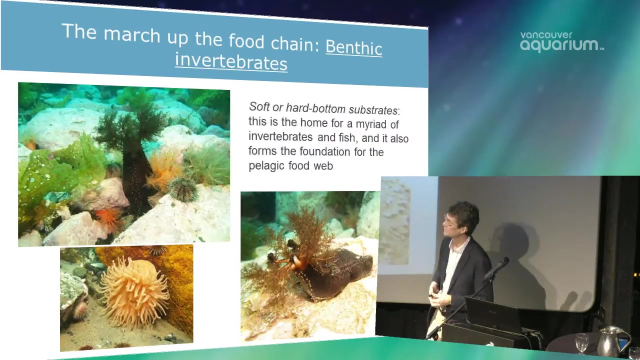 Others you'll find sitting on the top of the sediments or on a rock filter feeding, And a lot of these creatures form the basis for the entire food chain, upon which we will talk a little bit more in a second. So obviously some pretty spectacular creatures down there. 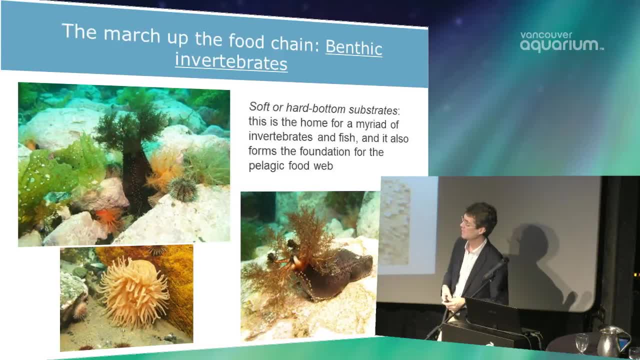 I believe that you'll hear more about that in another course from this series. But some wonderful sea anemones, sea cucumbers and other species, Very colorful, very vivid, And if you think about these species and the way in which they interact with their environment, 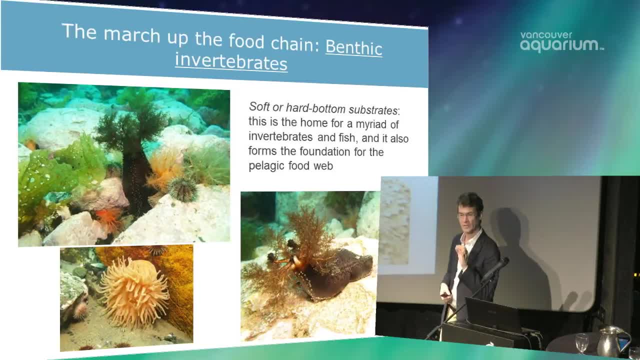 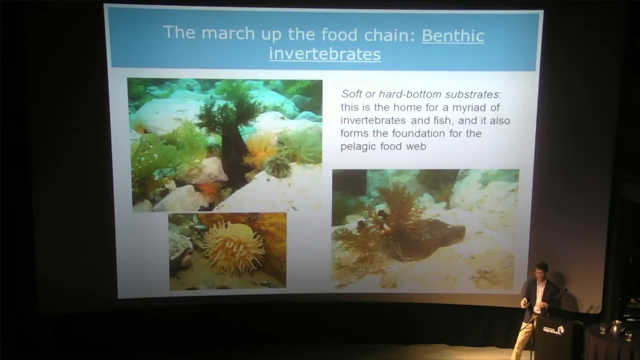 that's going to start to drive your ability to understand what kind of environment they might need. Do they need to attach to a hard surface like a rock, Just based on their lifestyle, Or do they want to move around with their feet and their claws and their various means of locomotion? 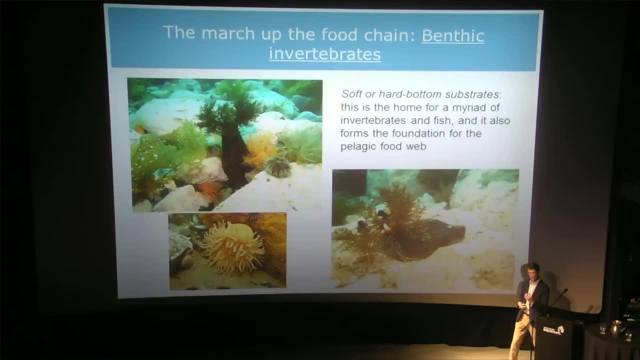 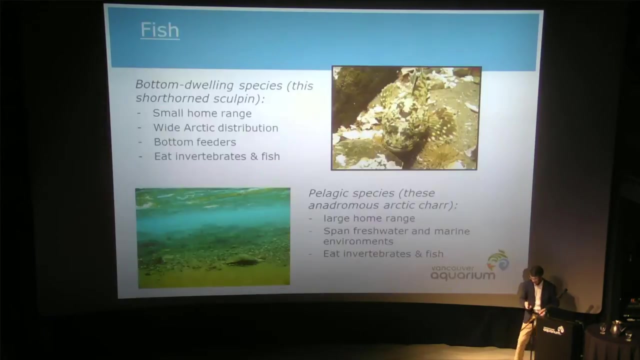 So understanding the way in which these species live, breathe, reproduce, move and feed is going to dictate where they're going to find a happy life and a happy home, And that's that interaction between the seabed habitat type or substrate type and the creatures you're going to find in those locations. 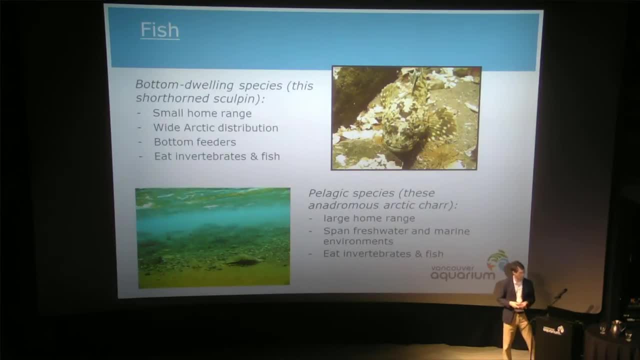 Of course, fish we tend to understand a little bit more than invertebrates, because we tend to have a lot more fish at the dinner table. We've got fish that rely on the bottom of the food chain and live on the seafloor. 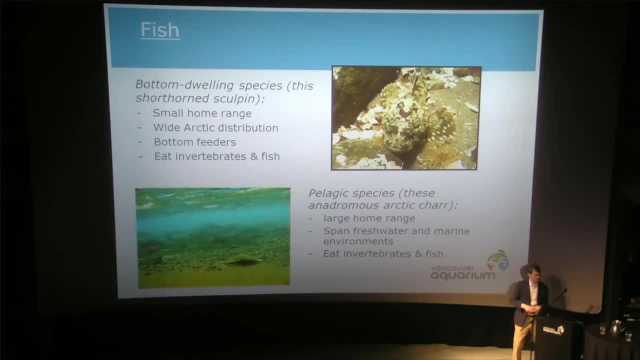 There are some flatfish In this case. we've got the example in the upper right here. this shorthorned sculpin, which is a resident fish, lives on the bottom, eats a variety of different species of both fish and invertebrates. 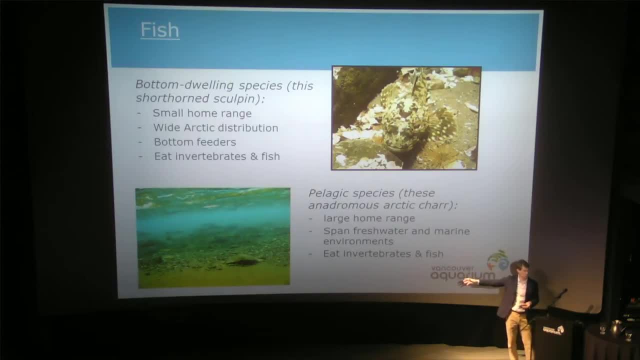 Pelagic species, of course. In this part of the world we've got Arctic char, which is anadromous. It migrates from freshwater into the ocean and then back again, just like the salmon here, And char is in fact a salmonid. 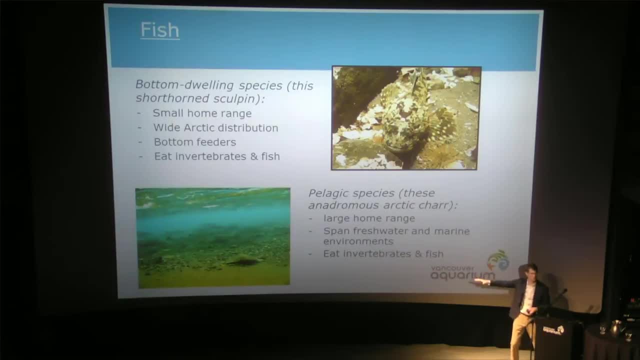 And this is something which is a little bit less connected to the sediments, But nonetheless they're still looking for food. They're still feeding on some of the same invertebrates and or smaller fishes that we'll find more connected to the habitat associated with the bottom of the ocean. 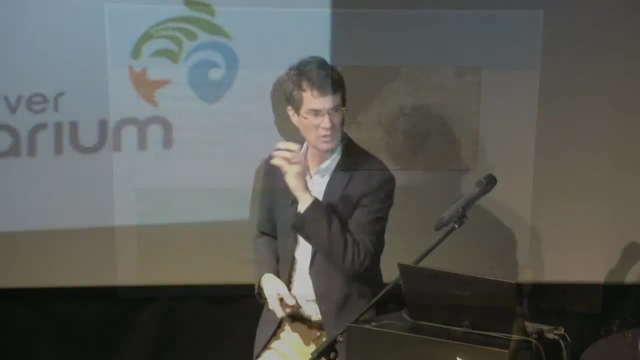 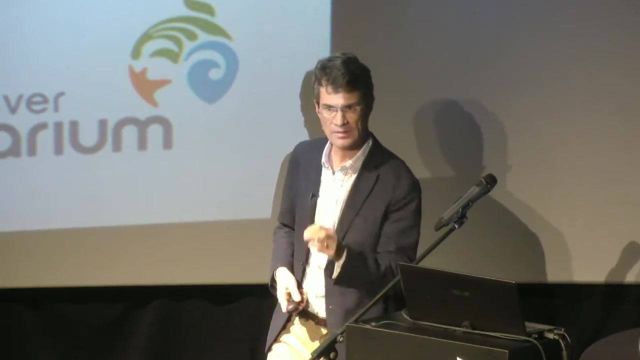 So even when we've got these big fish, these mobile species that are only transiently present in some of these areas, they're still in some way connected to that seabed and connected to the sediments and the benthic biota upon which the food chain relies. 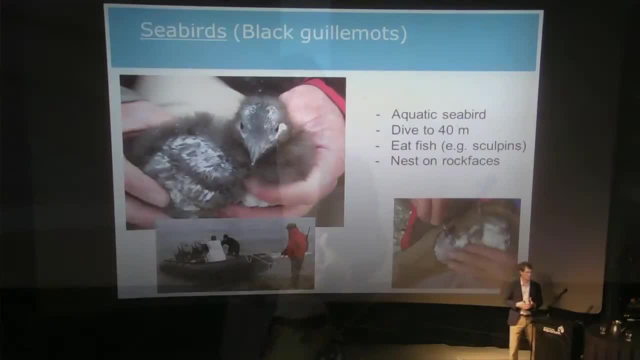 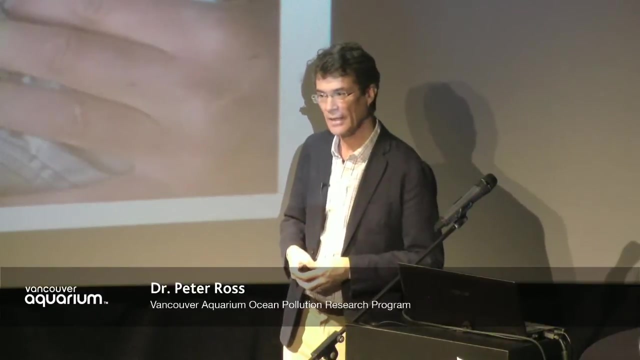 I'm going to go up the food chain just a little bit here. Pigeon guillemets. This is an aquatic seabird, largely localized, pushed around a little bit by virtue of their desire, essentially, to find food forage and live in coastal waters in Arctic areas. 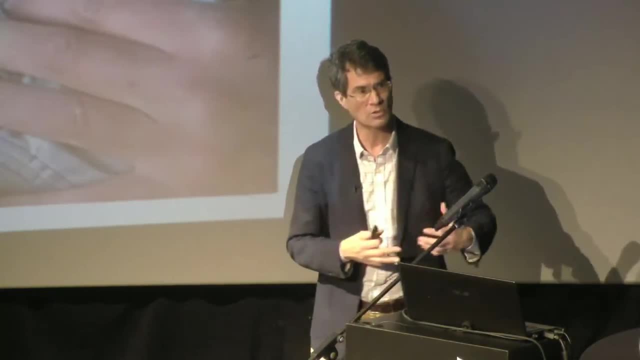 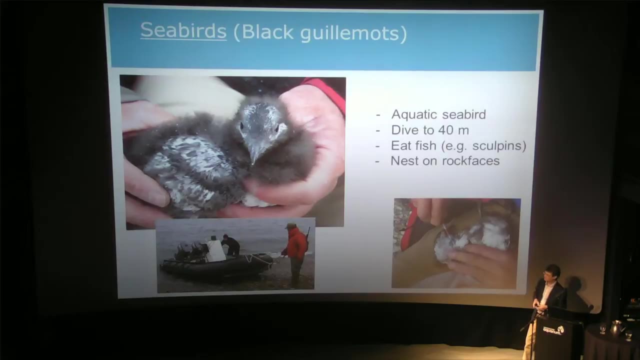 But of course, when the ice comes along, then they're pushed out of some of their local habitats. They're still going to be largely a resident of the Arctic environment. So this is a chick, And for parts of this research you can actually go out. 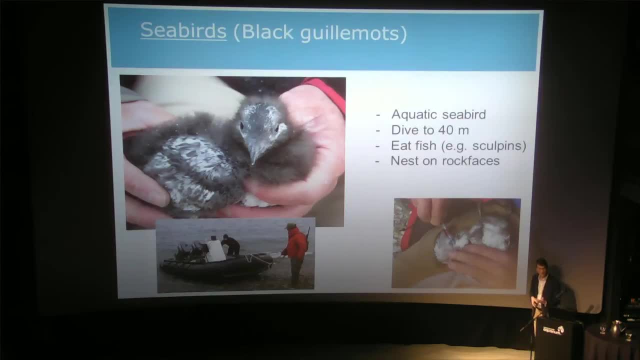 And we've got colleagues at the Canadian Wildlife Service that go out and sample these animals And then we can learn a lot more about them. We can learn a lot more about their feeding ecology, their physiology, their nutritional status and some of the anthropogenic stresses that we worry about. 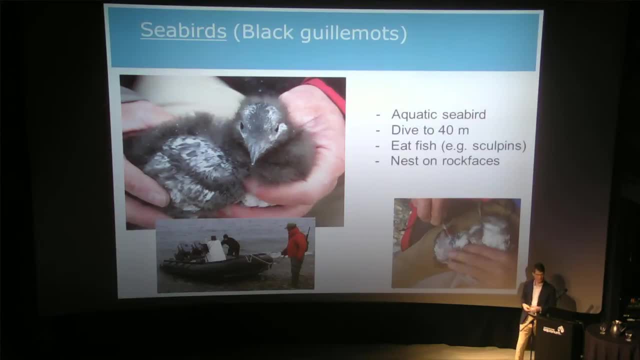 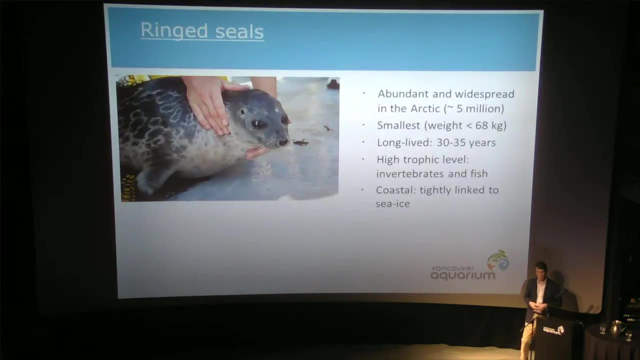 when it comes to top of the food chain, creatures like climate change, food availability related to climate change or global pollutants coming from multiple sources. Of course, the food chain would not be complete without putting a marine mammal at the top. I do like to talk about marine mammals. 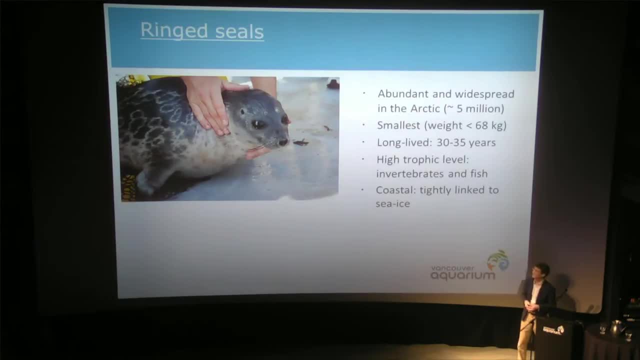 I've been studying marine mammals for almost 30 years. This is a ring seal. This species is very widely distributed throughout the Canadian Arctic. They're largely solitary. They don't hang out in big social groups. They're fairly small. They're long-lived, like most marine mammals. living maybe 35,, 40,, 45 years, And they really are very strongly associated with the ice edge And you might say, wow, okay, marine mammals, they swim. You see them on rocks, You might see them on ice. 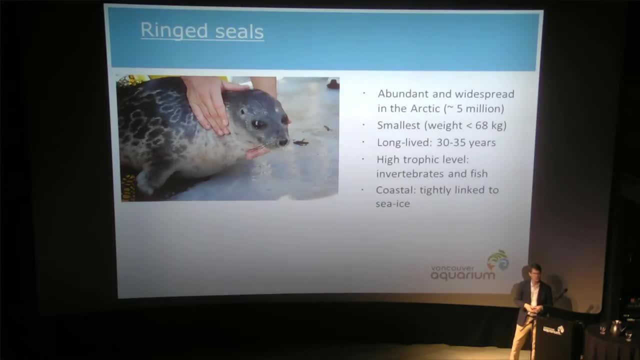 You might see them on the ice edge. What's that got to do with the sediments? So, as you can see, with the story that I'm providing for you this evening, we're going from the bottom up to the top in terms of the abiotic environment. 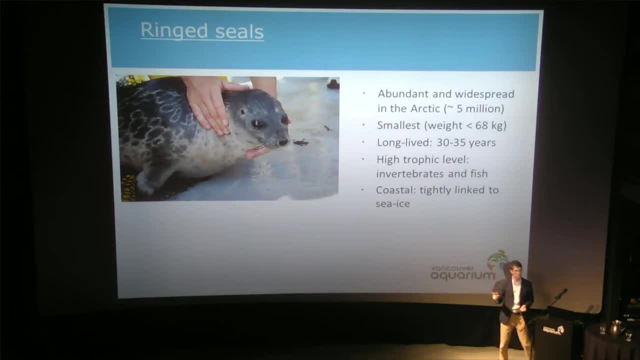 but also in terms of the biological environment. We're at the top of the food chain. now You might think that this creature is far removed from the bottom of the ocean, but in fact, it is connected to the sediments in a number of different ways. 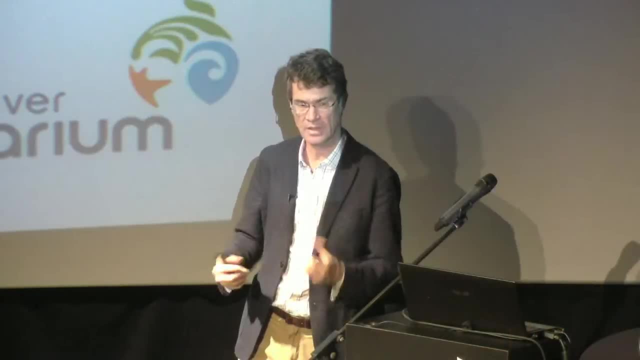 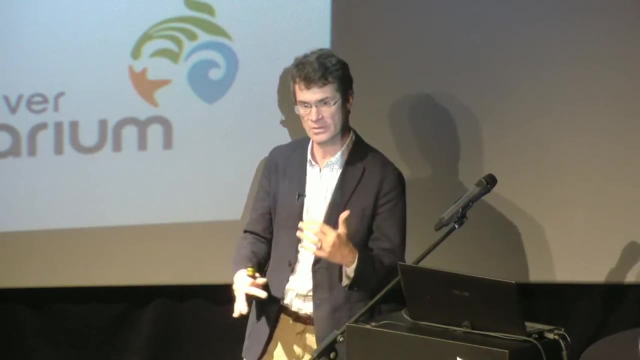 And, first and foremost, in terms of biological productivity. think about the sediments being the foundation of what's going on in coastal waters. Think about all the creatures: the polychaetes, the sea urchins, the isopods. 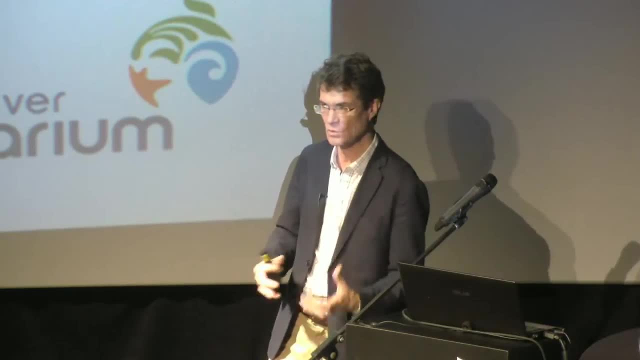 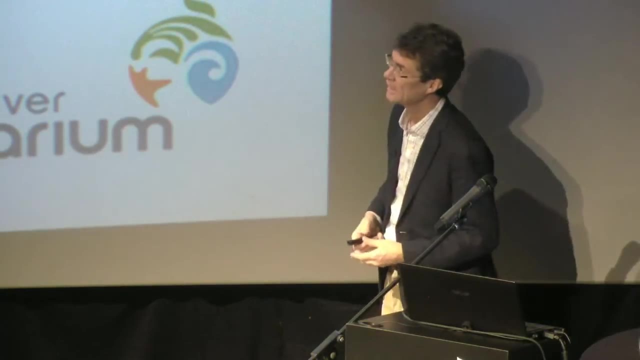 different invertebrates, different ground fish that are getting productivity associated with organic material in and around the sediments, and then think about that food chain, Then we're talking about a complete story which, in this case, we're going to call the Labrador Coastal Food Web. 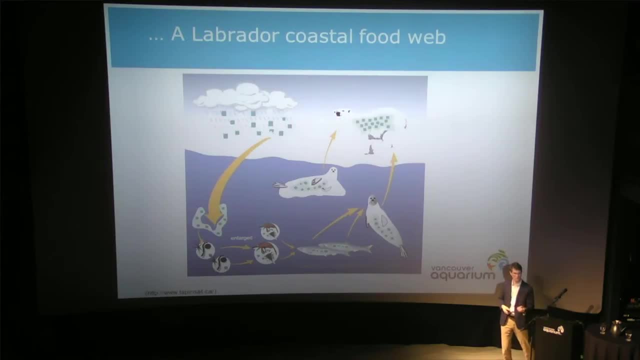 And, of course, a food web is a story about energy cycling, it's a story about carbon, it's a story about lipids, which is the currency of metabolism and growth, and it's also a story about pollution, and pollution is where I head next. 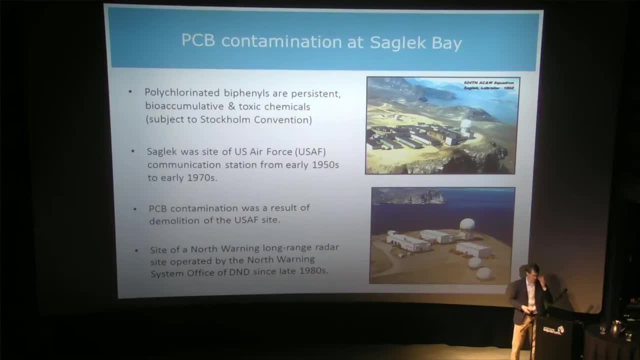 In this case. Sagalik Bay is a fjord in the middle of northern Labrador, along the coast, just at the border of Torngat Mountain National Park, and there was an accident here. Well, one might say it was deliberate. there was a spill of 450 kilograms of PCBs in the late 1970s. 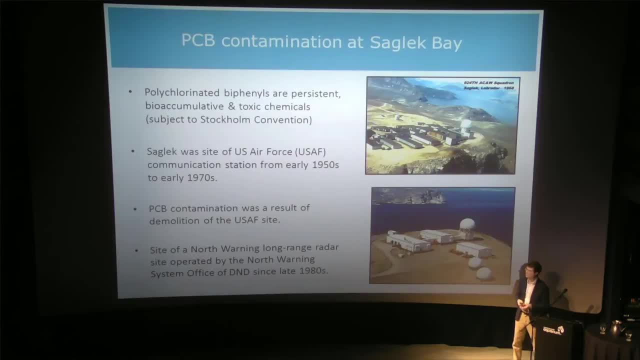 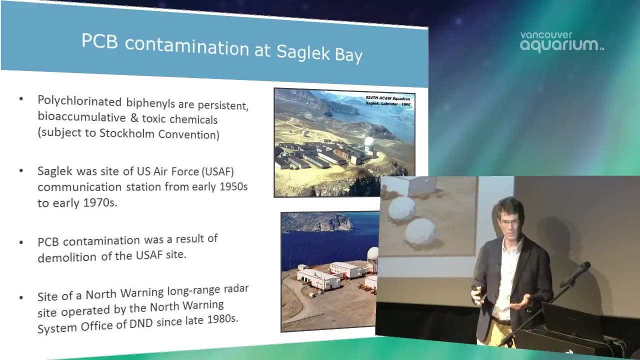 when the US Air Force was transitioning to a Canadian military radar station, and a lot of waste polychlorinated by phenols were bulldozed into the ocean as part of the cleanup effort. Unfortunately, out of sight is not out of mind. 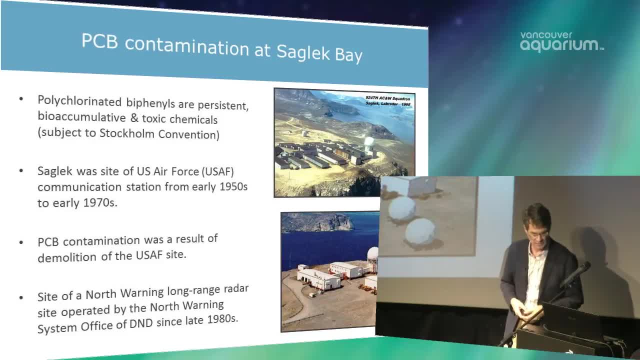 because this cleanup was not in fact a cleanup and it led to a legacy of pollution. The problem was associated with this very persistent endocrine-disrupting chemical that most people have heard of and, despite being banned in 1976 in Canada and, in fact, from much of the world, 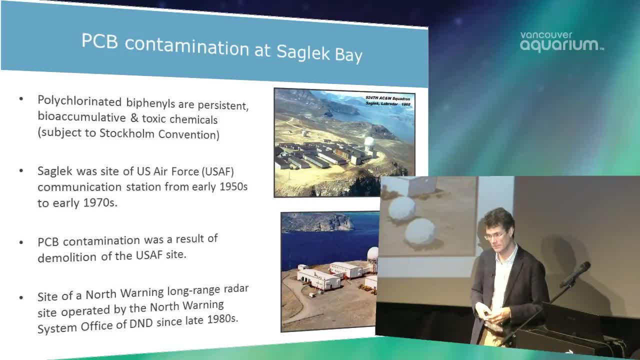 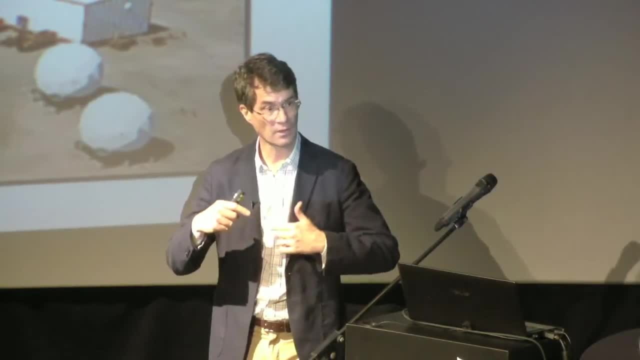 PCBs released in the 1950s, 60s and 70s are still out there cycling around, So we're waiting for them to break down, which is very, very slow, but we're also waiting for them to get buried in the sediment. 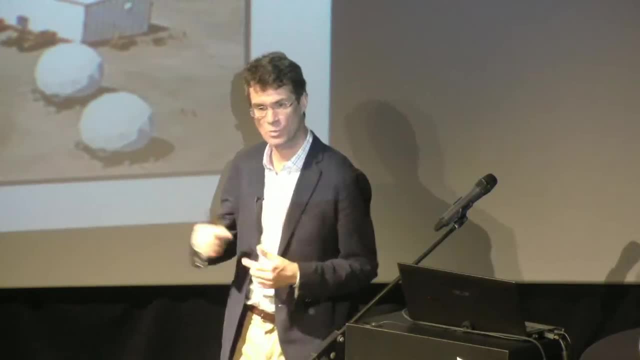 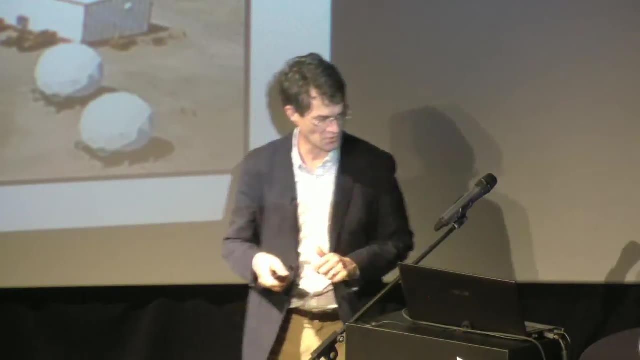 with natural sedimentation programs and chemical processes. That's the best we can hope for is that PCBs really get sedimented out and buried, so there's a cap on top of these old reservoirs of PCBs. So a story here about the Cold War as well. 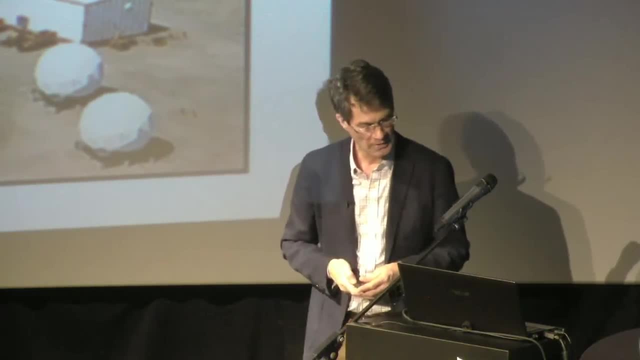 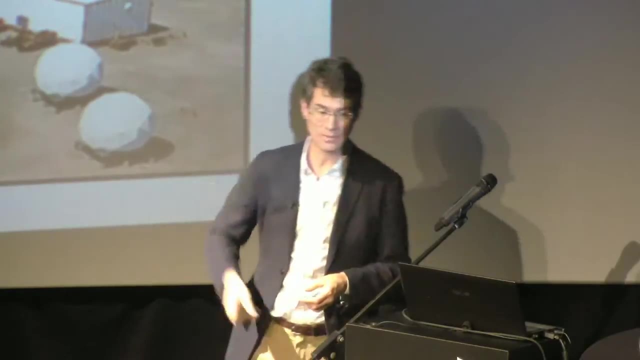 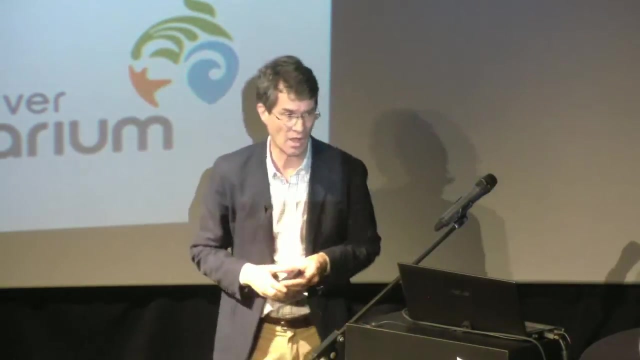 This was a radar station during the Cold War to warn about possible incoming missiles or aircraft and unfortunately the legacy is related to this toxic chemical spill And these are the sediment concentrations of PCBs. That's the highest concentration of PCBs in the sediments. 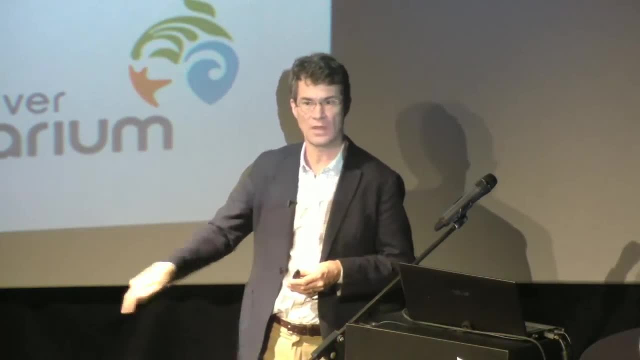 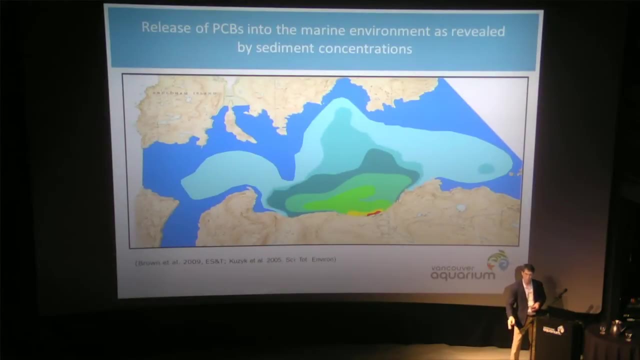 at the bottom of the ocean. Why are PCBs found in the sediments? It's because they are not water-soluble. And if they're not water-soluble, that means they're fat-soluble. And if they're fat-soluble? 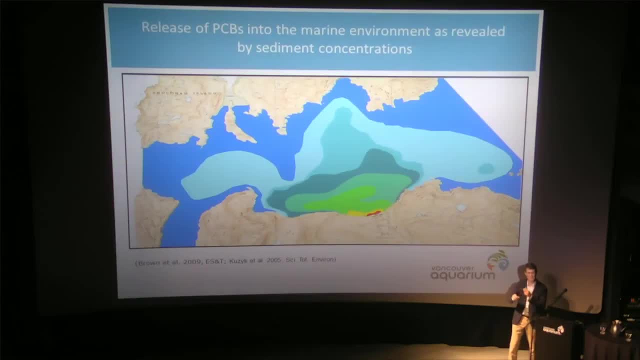 it means they're binding to organic particles and silt and little bits and pieces of grains of organic material and dropping out into the sediments. So fat-soluble, Fat-soluble, non-water-soluble chemicals like PCBs, like dioxins, like DDT. 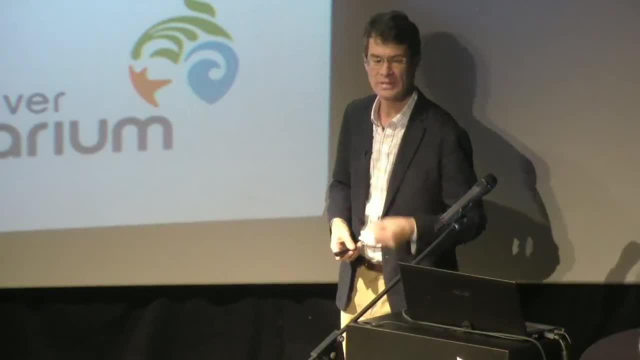 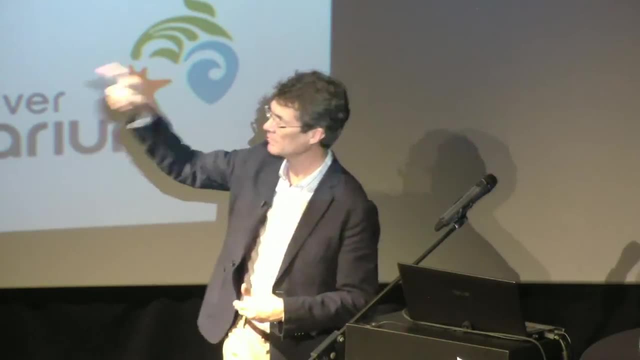 a lot of the old persistent organic pollutants, or POPs, that you may well have heard about. These things are all fat-soluble, particle-active. They bind sediment out. That's why you find them there And that's why we're worried about the food ban. 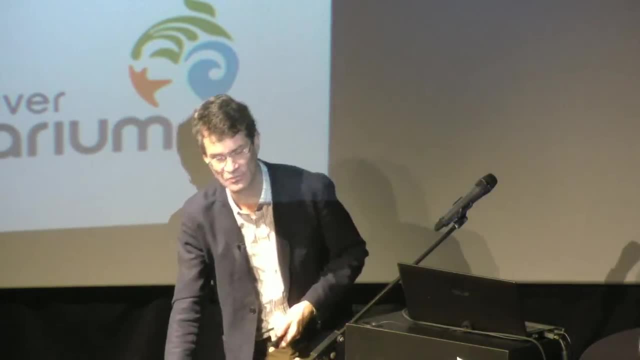 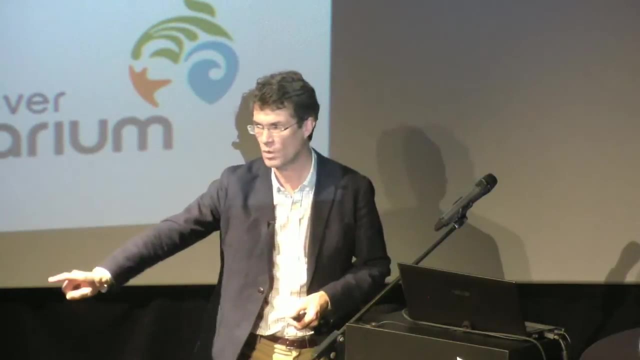 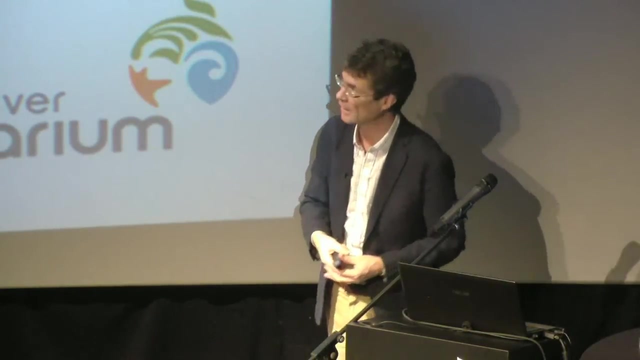 because if they're particle-active and dropping down into the sediments, the other place they can go is right into lipids, which means into algae, into bacterial cell walls, into the bottom of the food chain and up the food chain. because they're so persistent they're very difficult to metabolize. 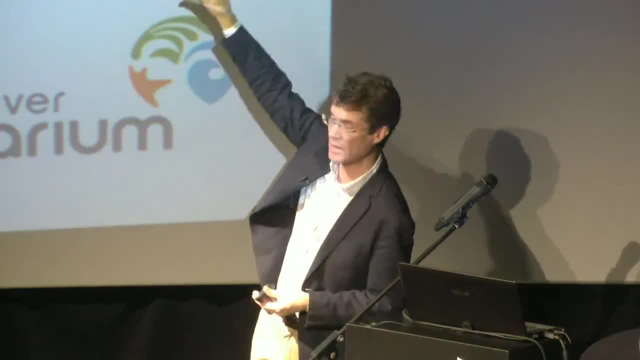 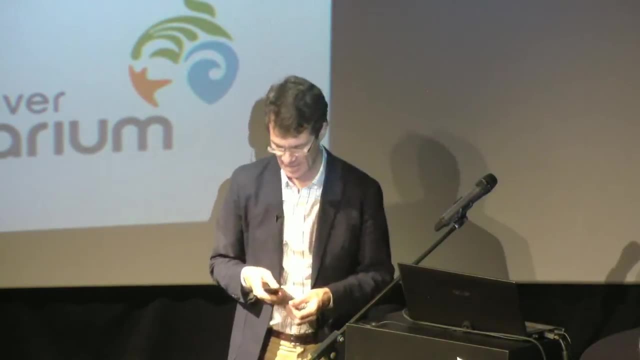 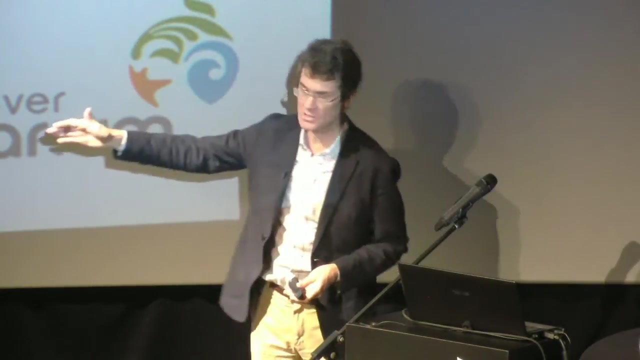 So this map gives you an idea of PCBs as they spread throughout this localized fjord, Seglek fjord, and contaminated vast stretches of this magnificent part of the eastern Canadian Arctic. And so what happens when we have high concentrations of sediment PCBs? 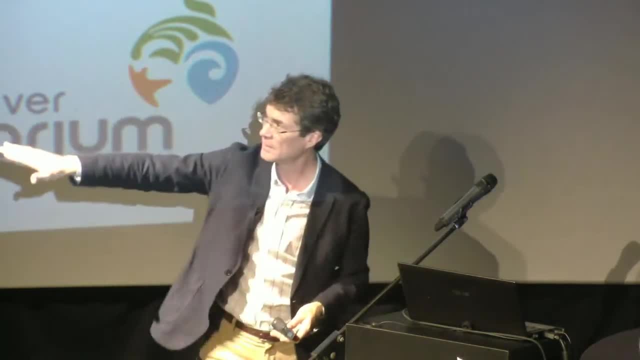 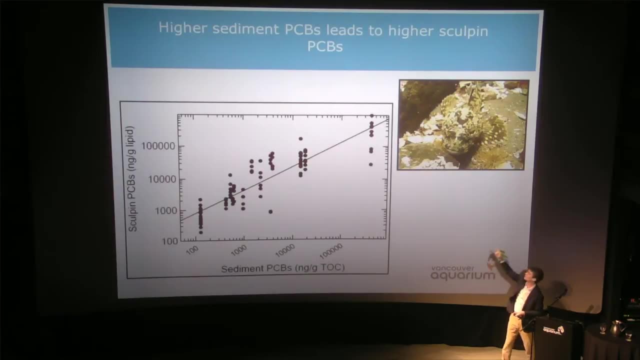 on the X or the horizontal axis, We see increasing concentrations in this fish, the shortfin sculpin. So a very distinct connection. This creature that lives at the bottom of the food chain and lives on the sea floor is not soaking them up through his or her skin. 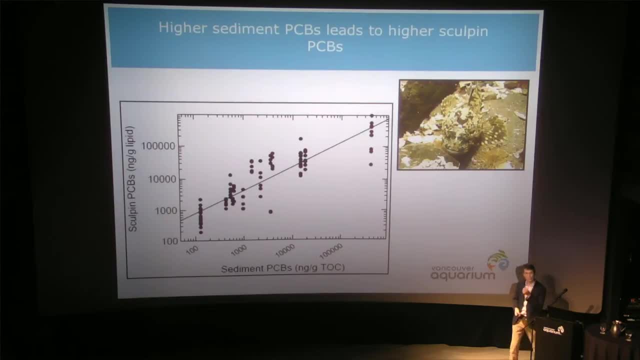 He or she is soaking these PCBs up from what it is eating largely So we have a very distinct connection. We have a very direct relationship between the sediment contamination and the contamination of the fish, such that the areas that have the highest PCB concentrations 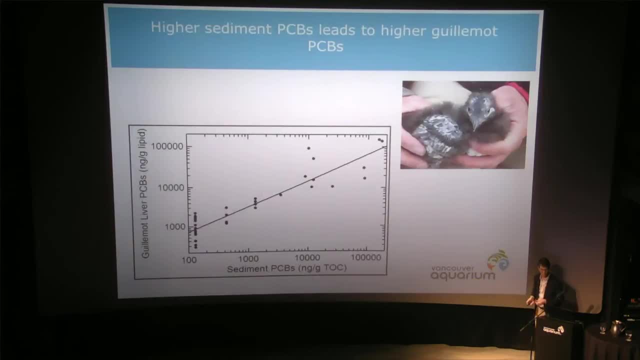 have the most contaminated sculpins. Very simple story. Here's an interesting one. We've got guillemets. These are birds living on the surface of the water, nesting on cliff faces, swimming around, paddling around. Same thing. 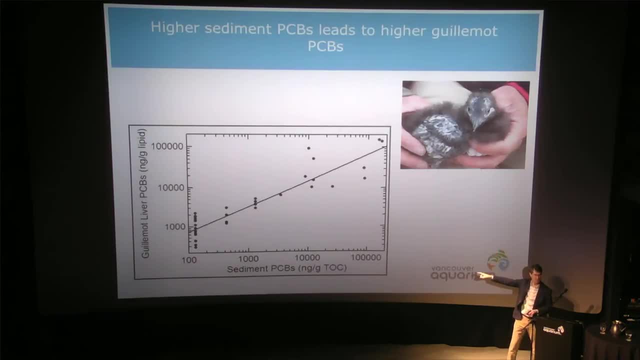 The birds that live close to the most contaminated sediment sites have the highest concentrations of PCBs. So another idea, another piece of evidence suggesting that contaminated sediments contaminate the food web and these PCBs travel all the way up to these higher trophic level creatures. 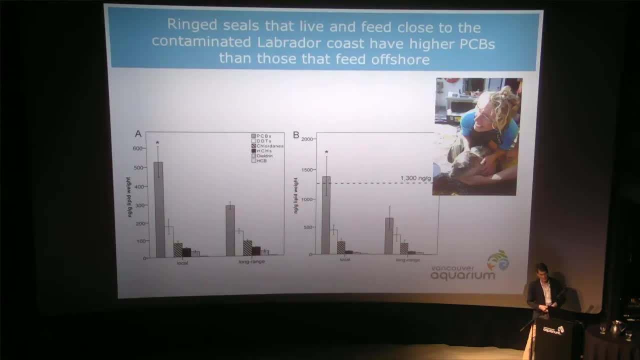 What does this mean for ringed seals? Well, ringed seals are much more mobile than the pigeon guillemets, so much more difficult to apportion blame, if you will. But in this case we were able to show that those seals 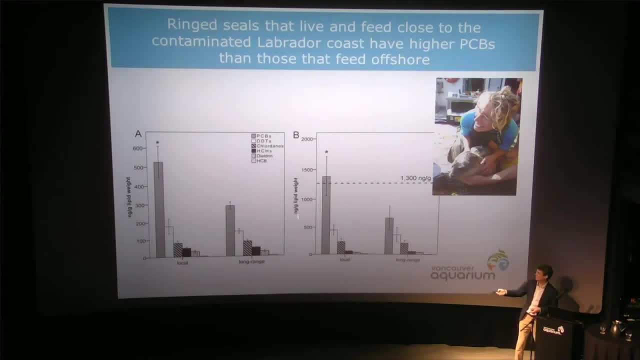 that inhabited local waters around the contaminated area and this tall bar here represents the PCBs in adults and the PCBs in younger animals living locally versus those that went and fed offshore in cleaner, more remote parts of the Northwest Atlantic Ocean. So much higher levels of PCBs in the seals. 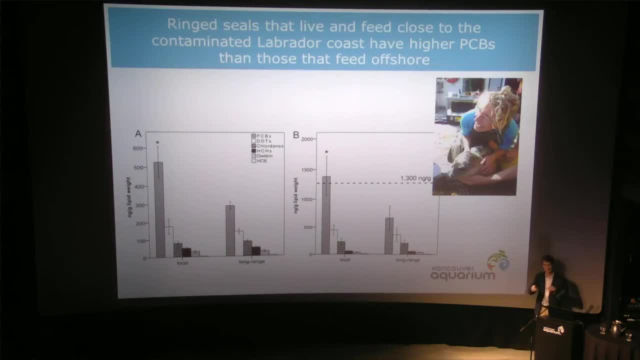 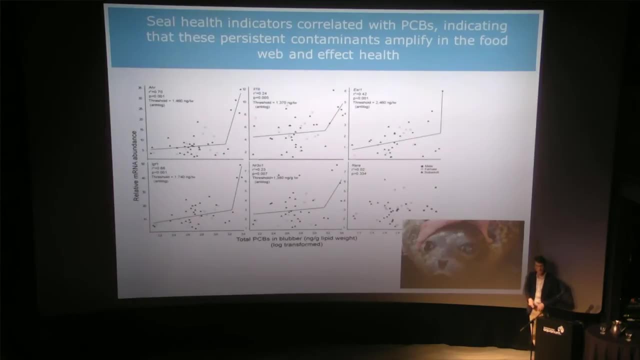 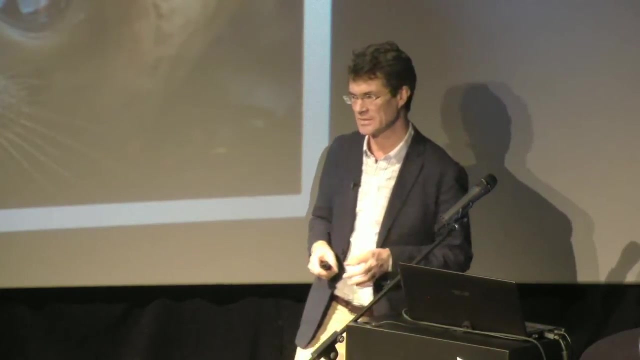 that are feeding in areas around the contaminated radar station. And we worry about PCBs, not because they're acute poisons, but because they're chronic, insidious endocrine-disrupting compounds or EDCs. They are hormone mimics. 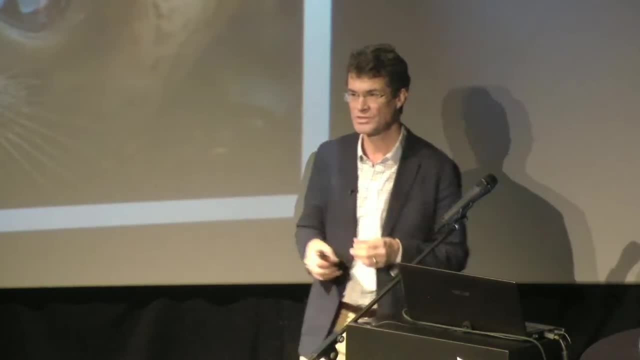 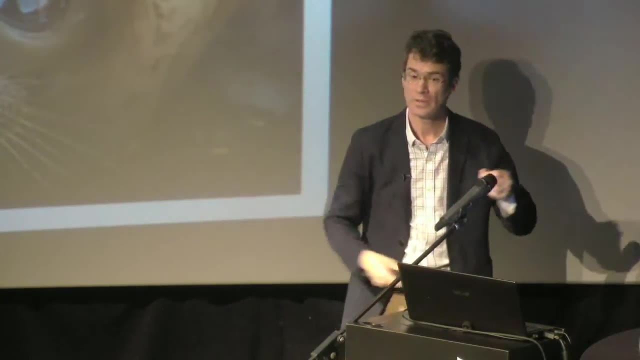 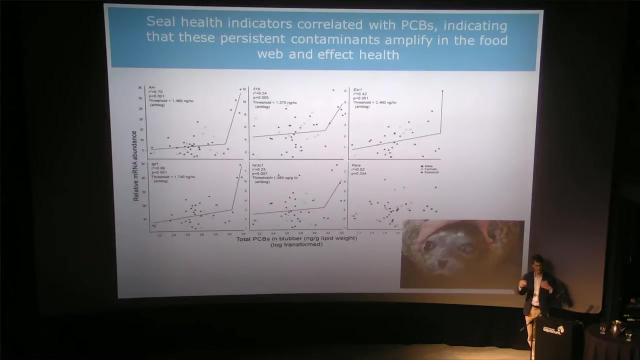 Some of the PCBs- there are 209 of them- resemble thyroid hormone and they can disrupt thyroid hormone physiology in seals and rats and humans. Okay, So endocrine-disrupting compounds- that's a catch-all phrase or term for a lot of these persistent chemicals that have been largely banned. 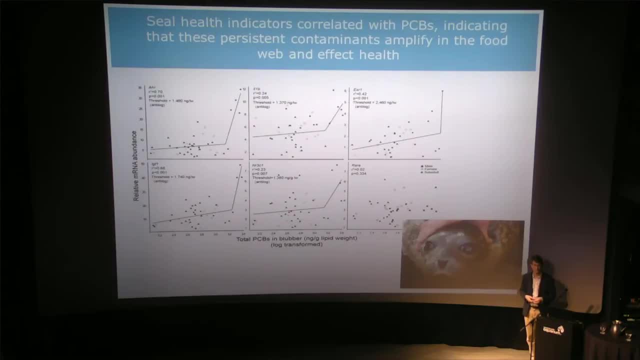 and those are the ones we call POPs, or persistent organic pollutants. There are other, newer endocrine-disrupting compounds that are less persistent, but we are nonetheless concerned about the potential for chemicals to disrupt growth, development and reproduction. You might have heard of bisphenol A. 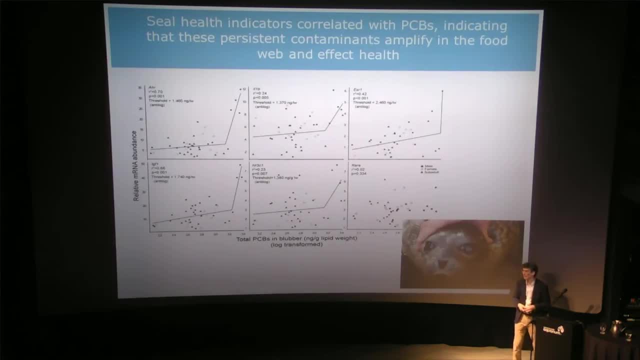 You might have heard of some other estrogen mimics. There are lots of them out there. But PCBs are these persistent chemicals that last for a long time out there, and what we see in these Herbert seals, based on some very high-end molecular work. 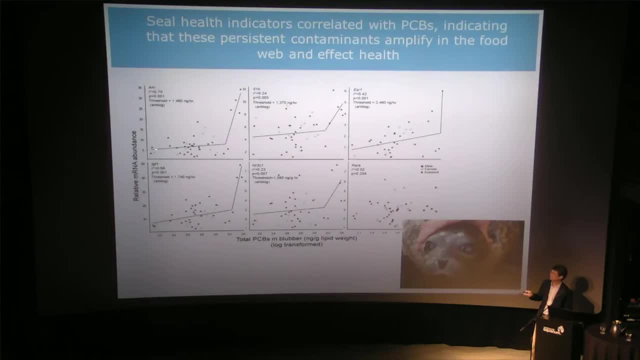 is. with increasing PCB concentrations, we see different genes being turned on, essentially being up-regulated here at about, well, at this dose, and it's about 1.4.. That's 5 milligrams per kilogram PCB. That's simply telling me there is a dose-response relationship. 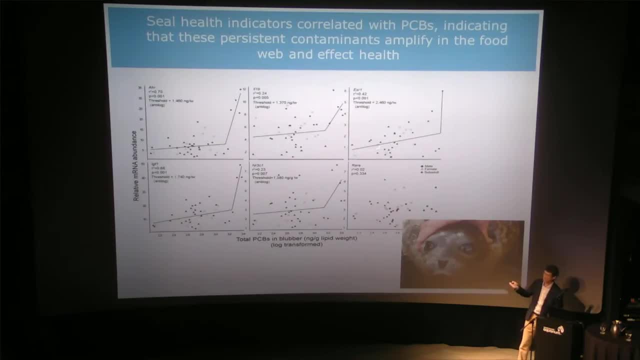 and a number of these- 1,, 2,, 3,, 4, 5 genes out of the 15 or so that we looked at- were turned on by exposure to PCBs, which means that PCBs in this locally contaminated area 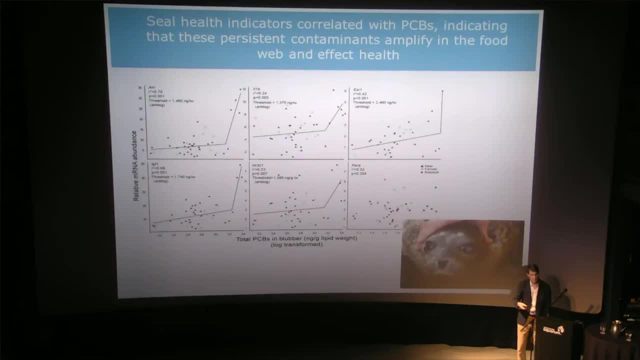 are contaminating the food web, leading to high levels in ring seals, and we're seeing molecular evidence of adverse injury or adverse effects. What this means to the health of the ring seal or the population more difficult to tell. This is molecular evidence. 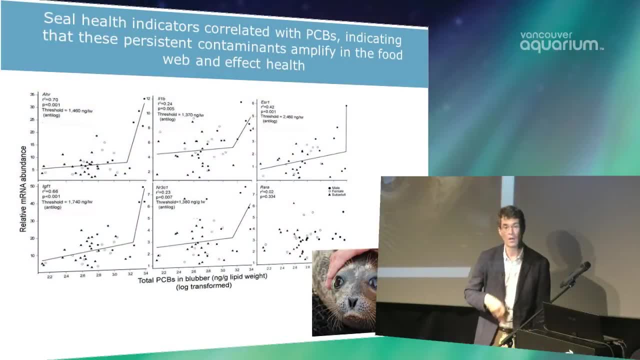 but what we do see in more contaminated areas are effects on reproduction, on incidence of tumors, on mass mortalities in marine mammals. We see a lot of evidence from much more contaminated marine mammal populations. Top of the food chain: contaminated ring seals. 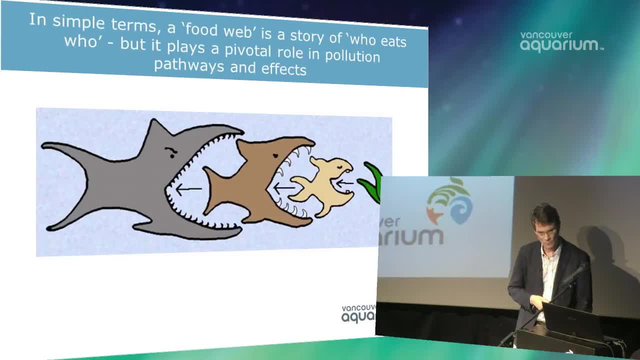 and consequence for their health. So, in very simple terms, tonight what I'm talking to you about is a food web or a food chain. Food chain is a simplistic view of things and that's what we've got right here. It's a story about who eats who. 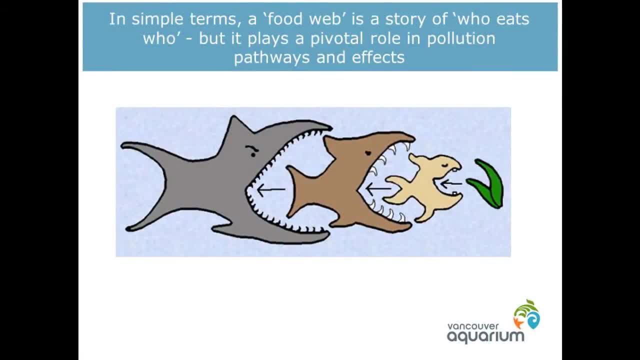 and this is a story about energetics and carbon and nutrients and the world around us, but it's also a story about pollution, and it's a story about some of these contaminants that do persist, that do bioaccumulate and are toxic at the top of the food chain. 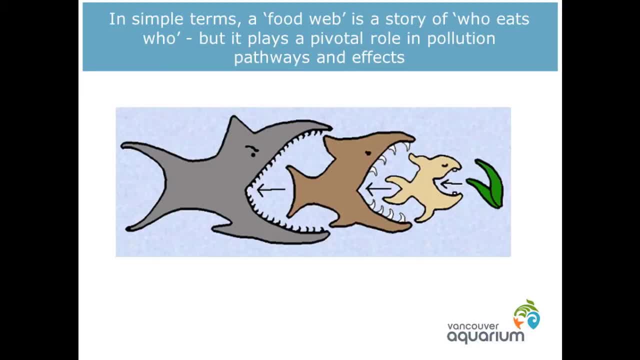 Those are the three words you ought to remember: P, B and T, persistent, bioaccumulative and toxic, because that's a generic definition of many hundreds, actually thousands, of different chemicals and that definition has a namesake in the form of the Stockholm Convention. 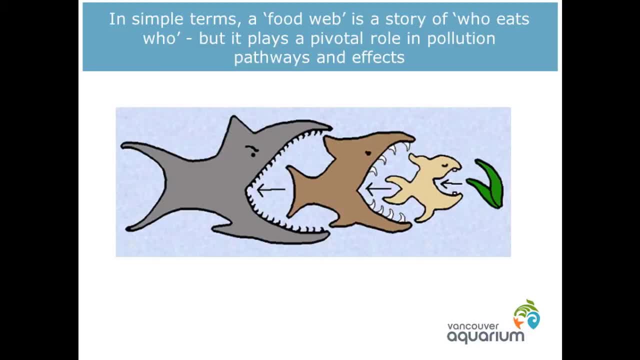 which is an international treaty to phase out and ban the priority persistent organic pollutants. Very important legal framework by which countries buy in and promise to phase out, regulate and take care of the environment by making sure they don't use these chemicals, because these chemicals have no boundaries. 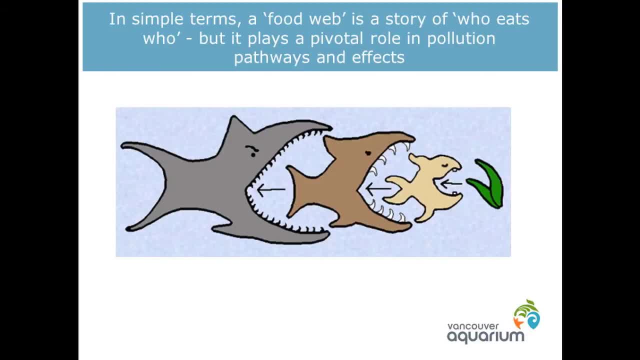 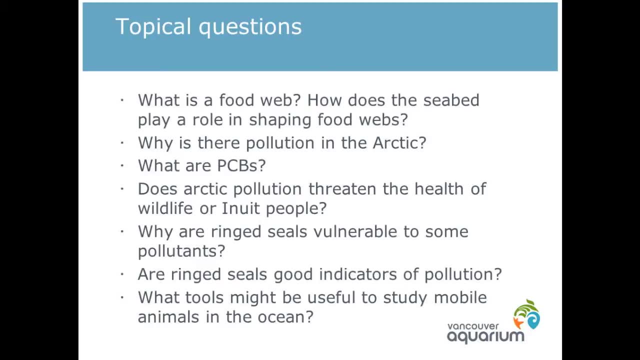 They end up getting into these food chains and they present problems to biota. So if you're thinking about what I'm talking to you about this evening, you might have a few questions in your head. I'm touching on an awful lot of different topics. 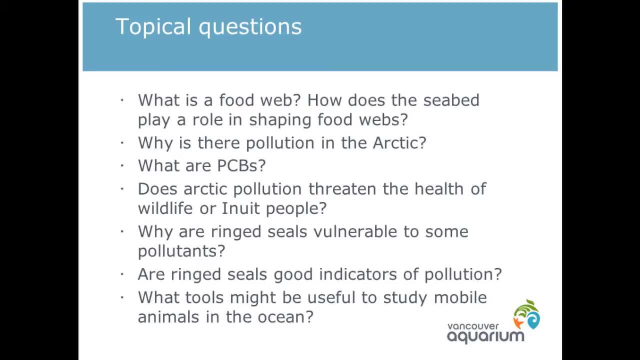 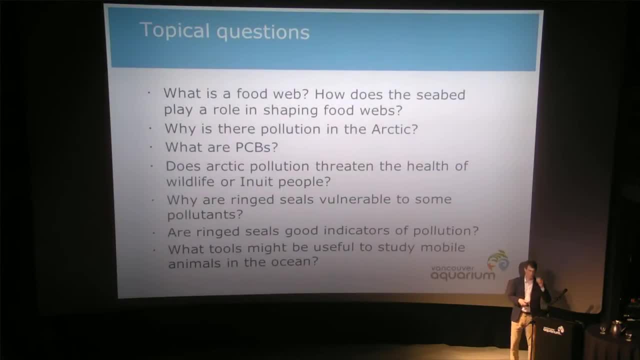 and an awful lot of different disciplines, a lot of different topics. Each of these topics, each of these slides that I described this evening and spoke to this evening has a very rich compendium of literature, of works of knowledge that speak to such things as: 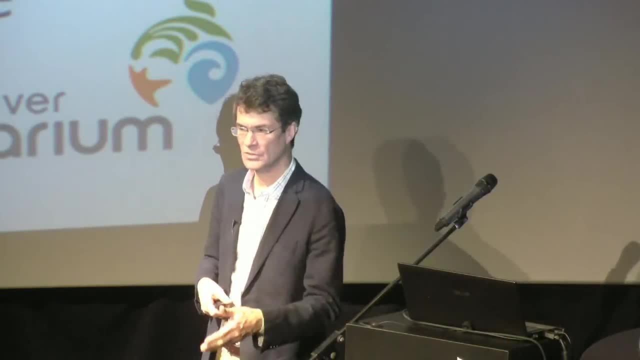 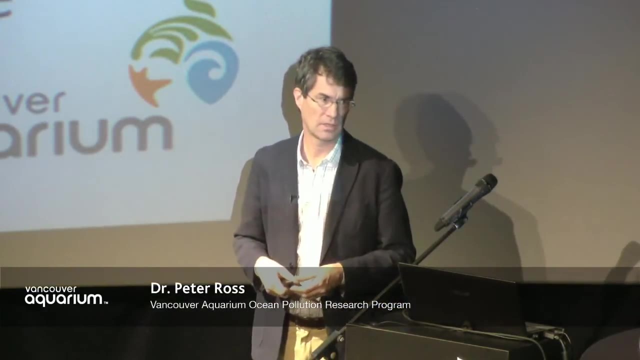 biogeography, physiology, toxicology, marine biology- a lot of different things going on here, So these questions can perhaps guide you in the right direction if you're looking to drill down just a little bit more, to understand a little bit more. 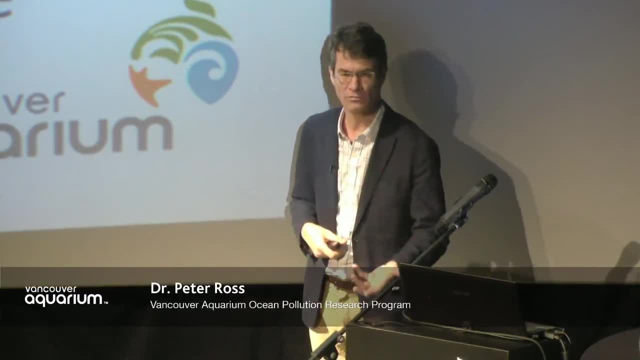 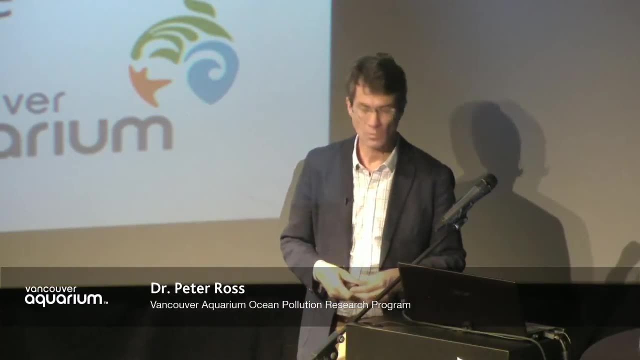 about what I've spoken to you this evening, And some of those questions would be related to food webs. What is a food web and what is the connection between the seabed and sea life? on top of that, Why is there pollution in the Arctic? 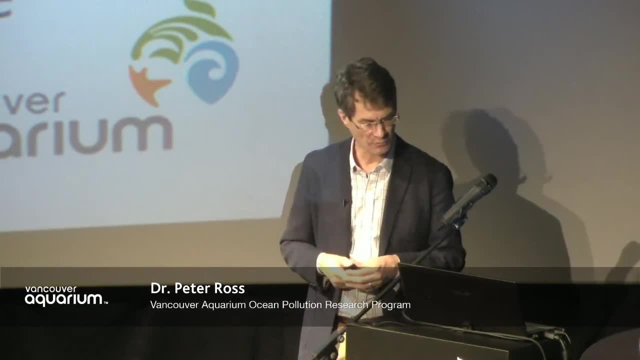 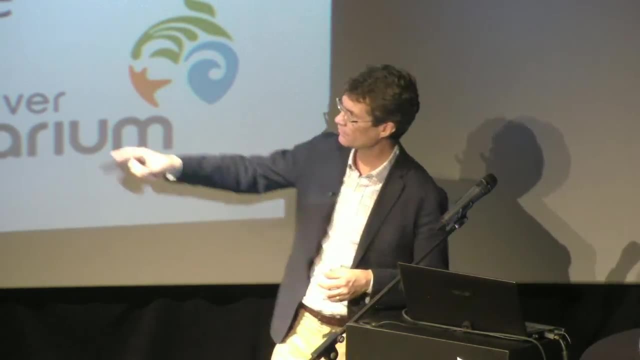 Why do we find pollution in the Arctic? Does it threaten wildlife or Inuit? Why are ring seals in particular vulnerable to high levels of these pollutants? And lots of questions here about tools. How do you study, How do you carry out research in the Arctic? 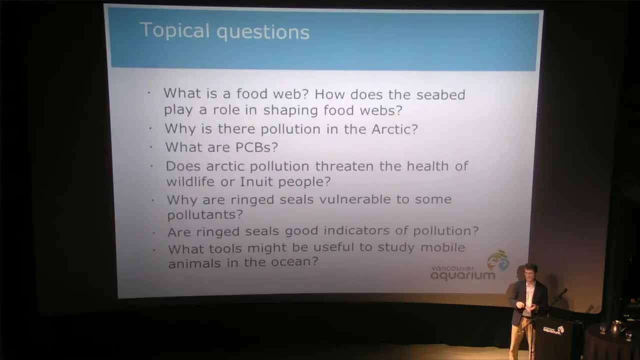 where it's tough getting into your study sites. The weather can be very challenging, The environment can be challenging. There's not much in the way of logistical support. You have to bring all your supplies with you safely and you can't forget anything. 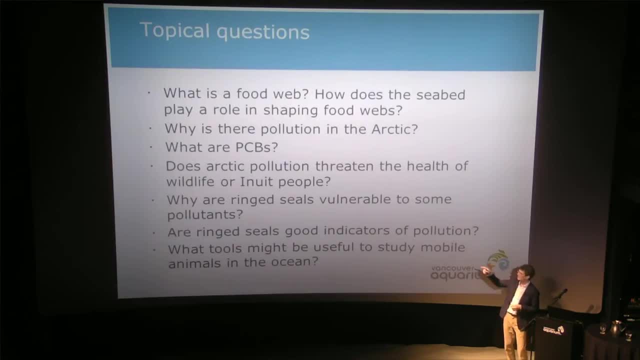 otherwise you're going to be caught off guard. So what kinds of tools might be useful to apply to Arctic research And, in particular, if you're trying to understand something about mobile species, either anadromous fish or migratory birds? 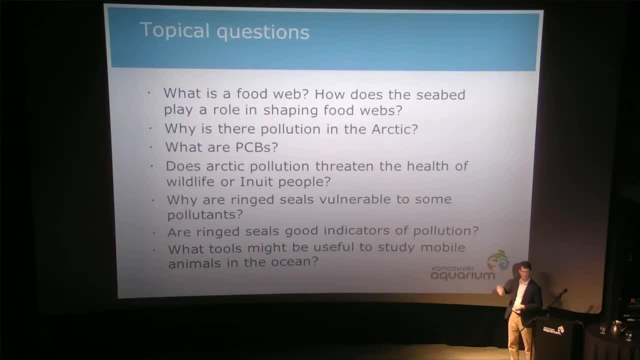 or seals that may move along with the ice edge. how do you actually do that? And once you start thinking about some of those questions, there's a wonderful body of literature out there that can shed light on some of the interesting tools that have been applied with success. 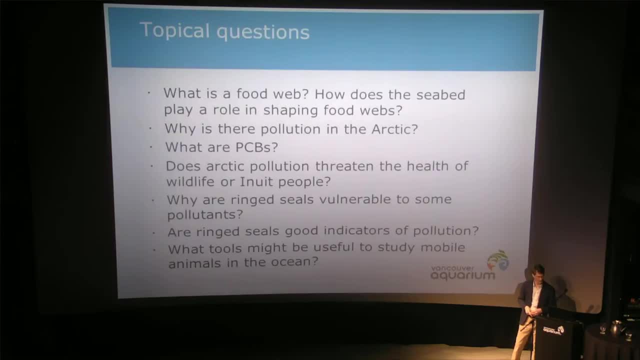 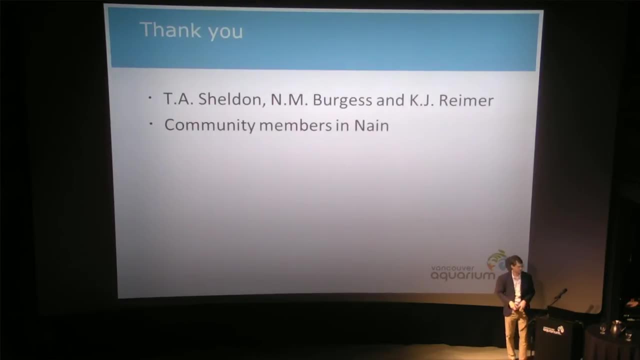 to generate stories and insight about the Canadiens. So thank you for your time and I look forward to any questions you might have. All right, thank you, Peter. So let's go ahead and take some questions from the audience And, Peter, maybe what you could do. 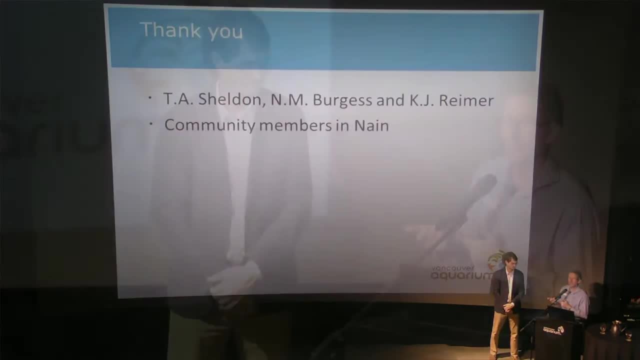 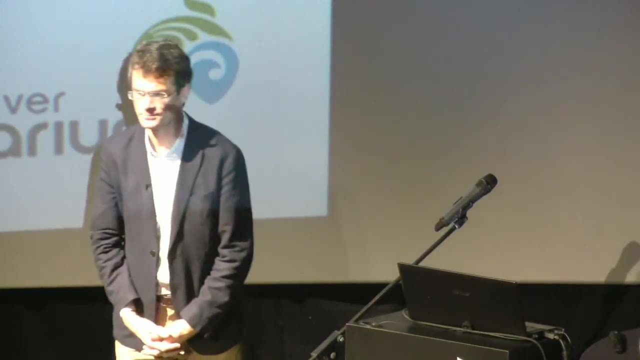 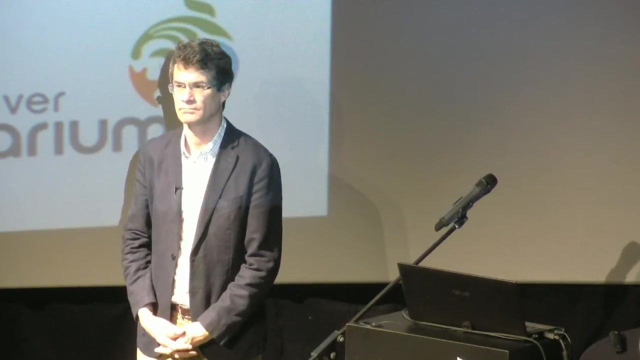 is just repeat the question so our online audience can hear it. So if anyone wants to go ahead. So some of the genes that are being upregulated. let's look at an example of one of the ones that were turned on. So the question was: 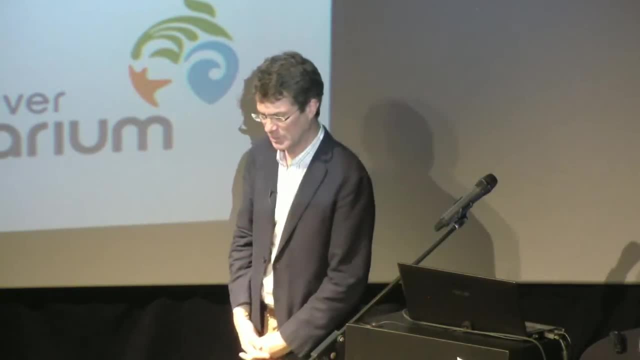 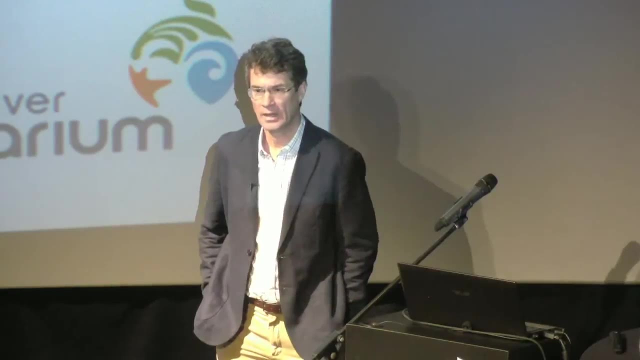 what are some of the examples of genes that were turned on by exposure to PCBs in this case? One of them is called the aryl hydrocarbon receptor, AHR- Aryl hydrocarbon receptor. we don't know a lot about it. 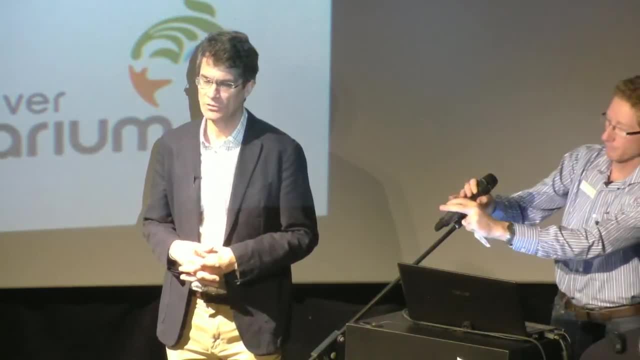 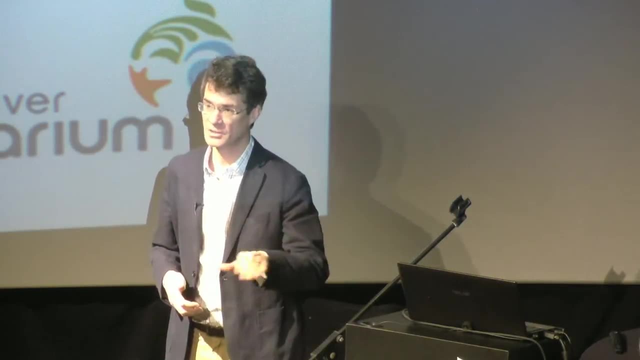 but all mammals have the AHR And in all mammals studied, what we see with the AHR is induction. So whether you're a lab rodent exposed to dioxin, or whether you're a heavily exposed human, we will see the AHR turned on. 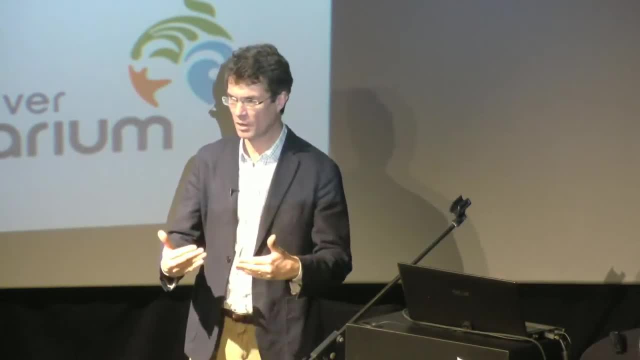 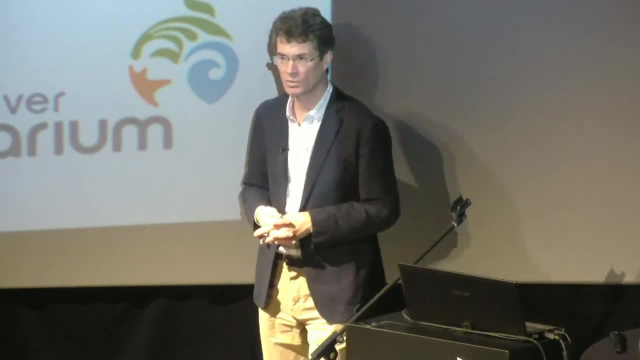 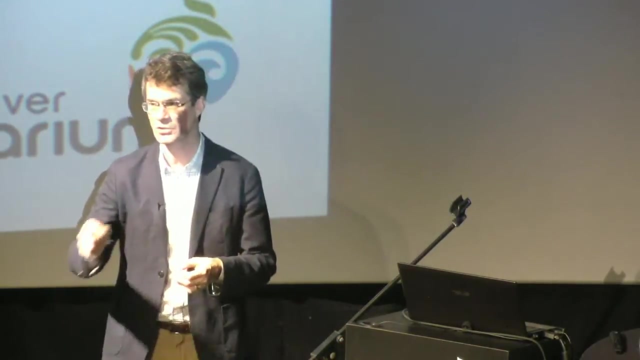 So it's typically viewed as a very defensible biomarker of exposure to dioxin-like contaminants, including many of the PCBs. That was one of them. Another one was the estrogen receptor. You might have heard of estrogen before, So to have the estrogen receptor turned on. 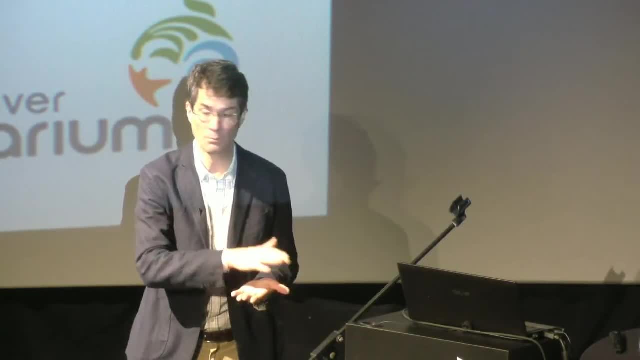 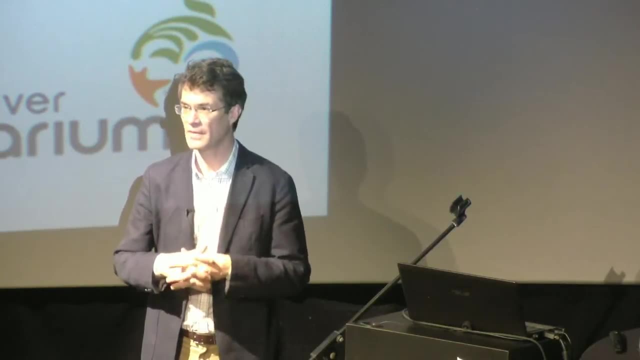 by exposure to PCBs, which we've seen in killer whales here in British Columbia, which we've seen in harbor seals here in British Columbia, which we've seen in other species, is troubling because that speaks to the potential for something like PCBs. 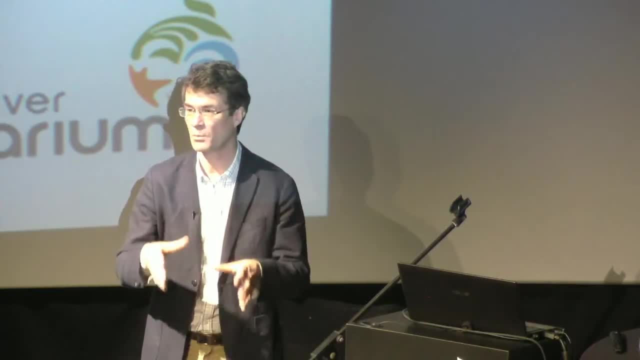 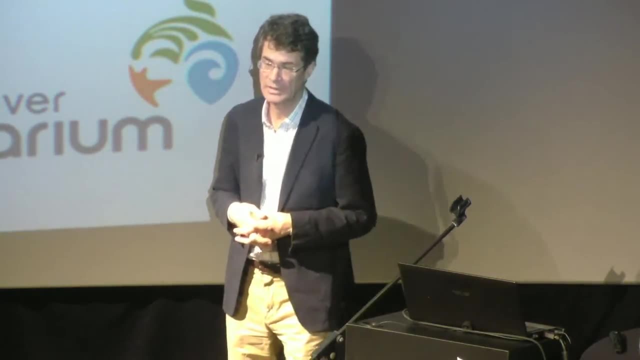 to affect the development of a healthy reproductive system in either males or females. So it's that sort of result that we tend to worry about With humans. very difficult to study these things because we've got a lot of confounding factors, very complex diets. 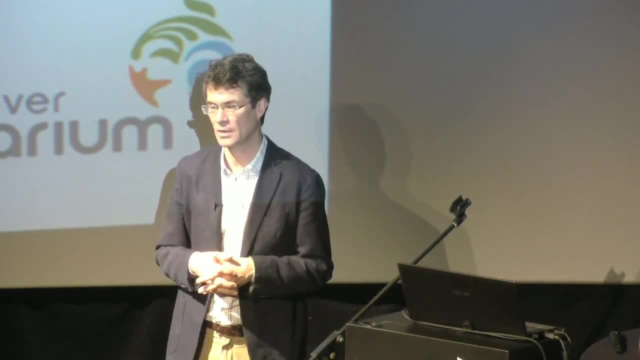 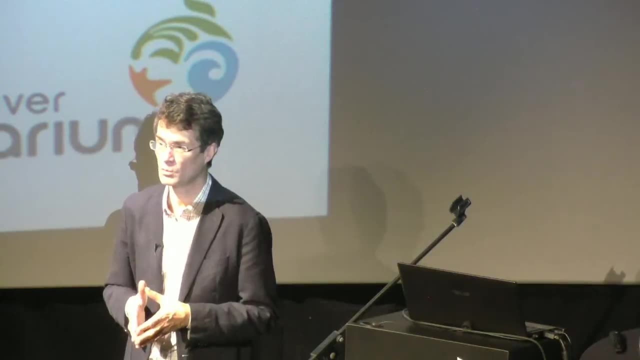 various backgrounds in terms of what we do and what our habits are, But those are two examples of genes that were turned on. Third one was thyroid hormone, Thyroid hormone receptor and, of course, you know what thyroid hormones are: very important for metabolism. 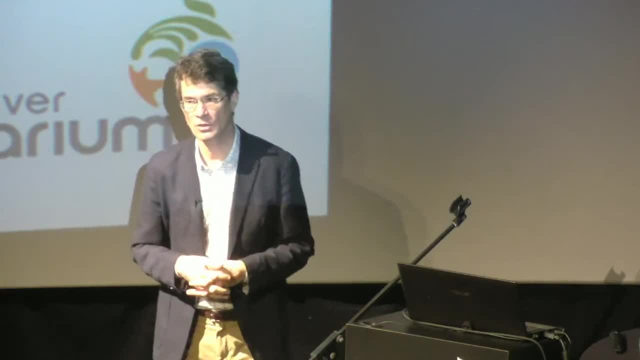 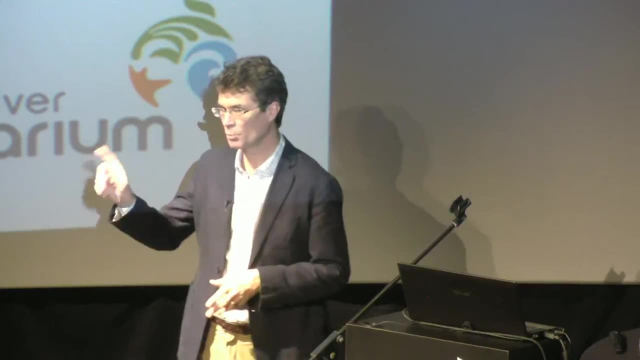 and growth and development. That is another gene endpoint that has been routinely turned on by exposure to moderate to high levels of PCBs. I should point out, though in all of these cases the doses were relatively low With these ringed seals. 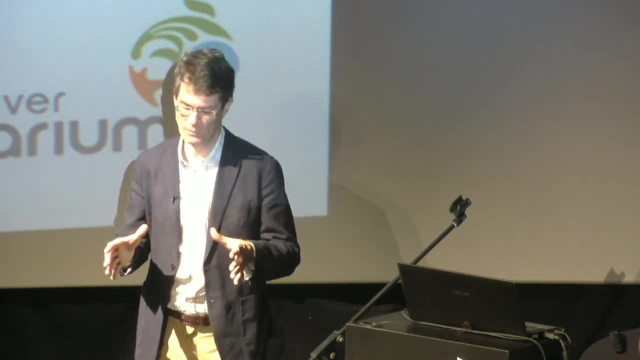 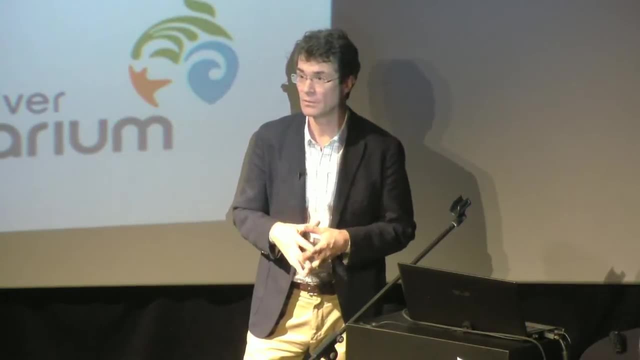 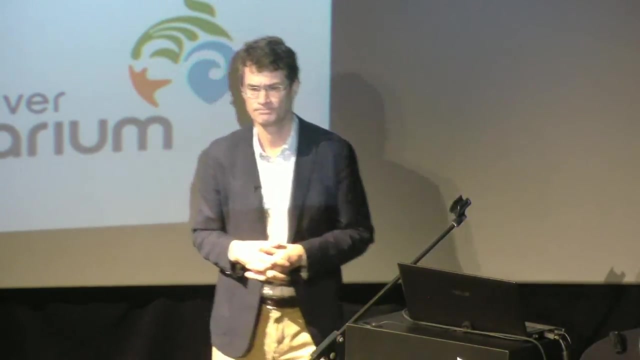 they probably have a concentration of PCBs that on average would be two to four times higher than the average Canadian human. So relatively low by our standpoint and certainly relatively low compared to a lot of other marine mammals in southern Canadian waters. How common are PCBs? 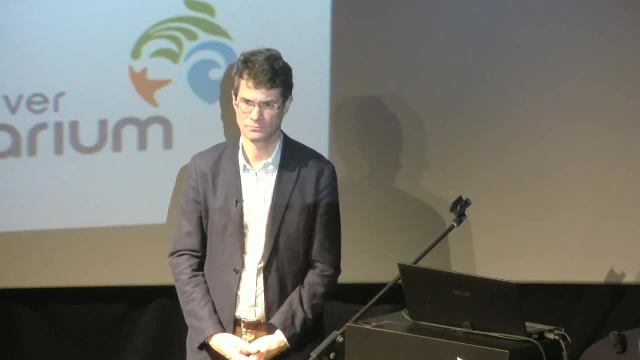 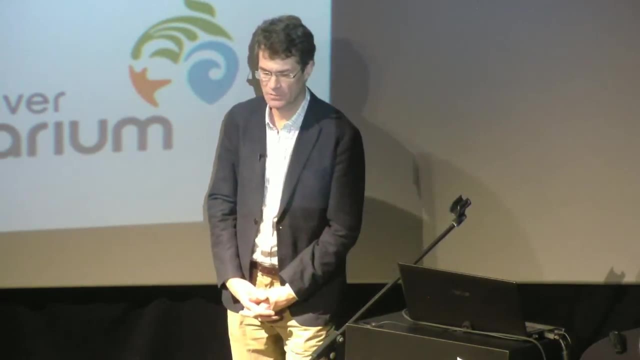 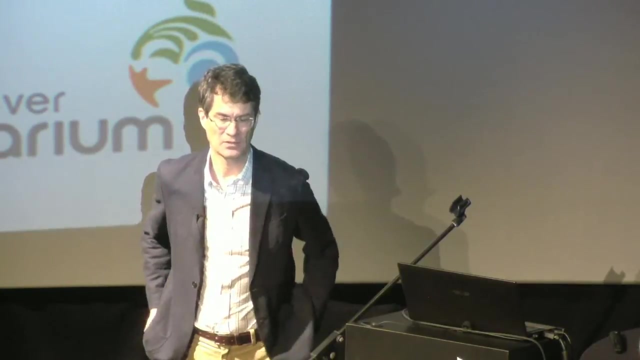 outside of Arctic waters? Do we know that? Do we measure that, Like in the effluent of the Fraser River? So how common are PCBs outside of the Arctic? Very common, PCBs are everywhere. They were used extensively between 1929 and the mid to late 1970s. Because they're so persistent they don't break down. They basically cycle around the world. They move through. they move through the atmosphere to remote areas. We find them, of course, throughout BC, Our resident and transient killer whales here in British Columbia. 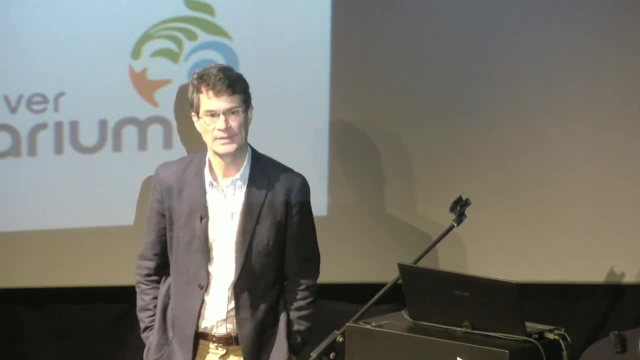 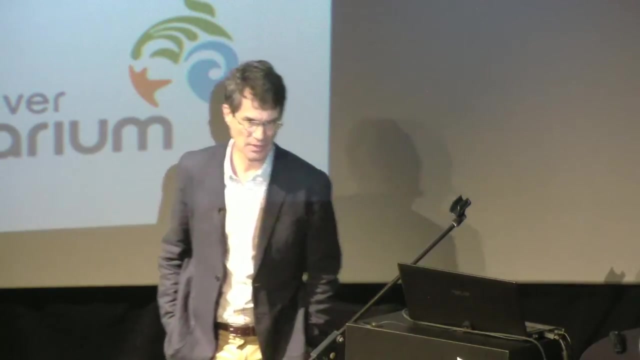 are some of the most PCB contaminated marine mammals in the world And we're watching the concentrations of PCBs decline. Since regulations in the mid 1970s in Canada, we've seen a decline in PCB concentrations such that harbor seals probably have one fifth the concentrations in BC. 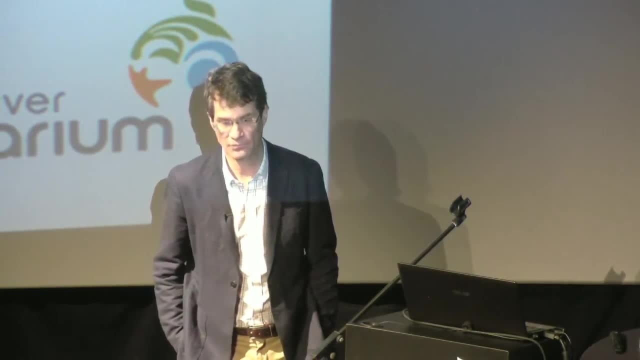 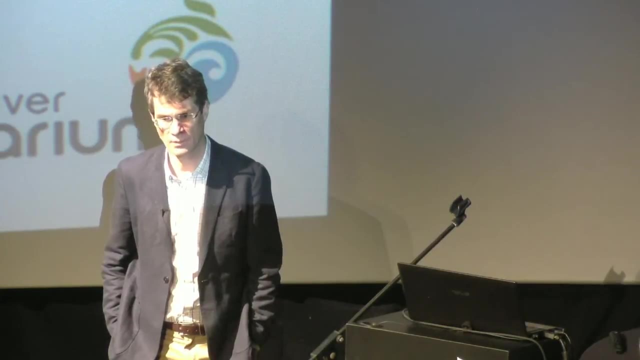 that they did 30 years ago. So we have been watching these declines, But PCBs do persist and continue, And the more we learn about them, the more we recognize that they were a threat that had to be addressed from a management and source control perspective. 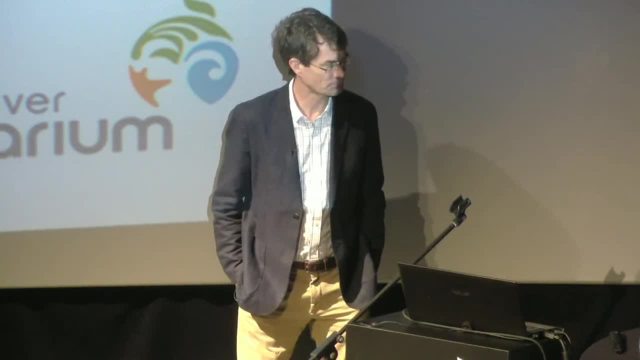 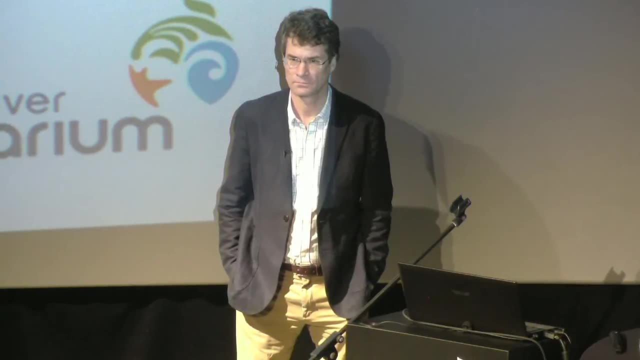 We have a couple of online questions, but I just I need to get them. So if we could take one more question here and then I'll get those two questions, Got another one Great. What were the PCBs being used for? 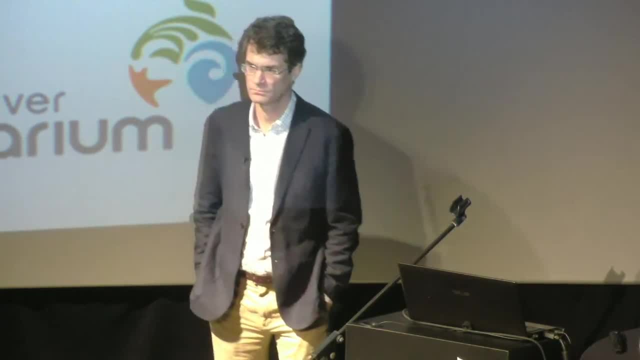 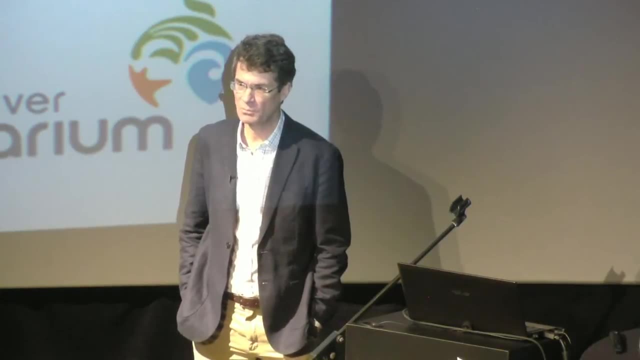 at the radar station. What can you mean by that? So what were the PCBs being used for at the radar station? PCBs were used extensively in urban areas with transformers, with electric transformers. PCBs are basically a very thick oil, industrial oil. 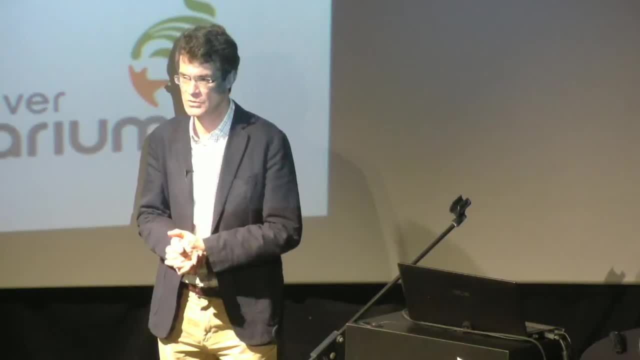 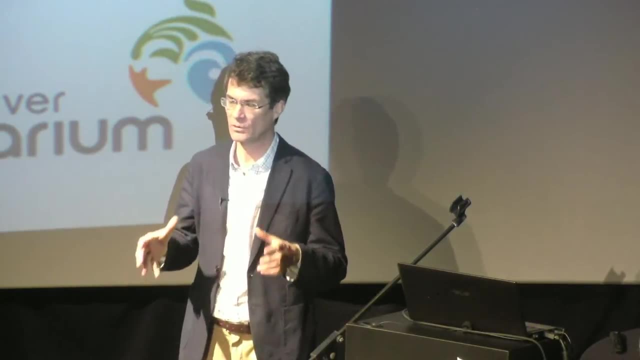 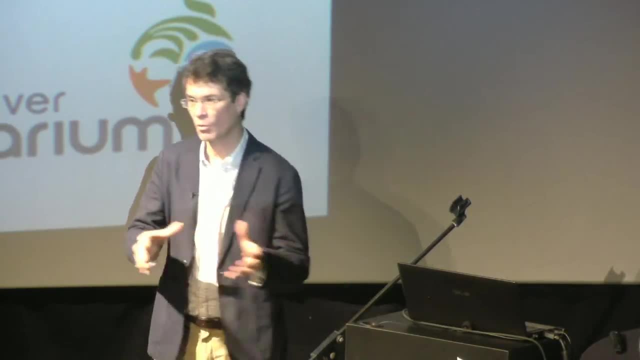 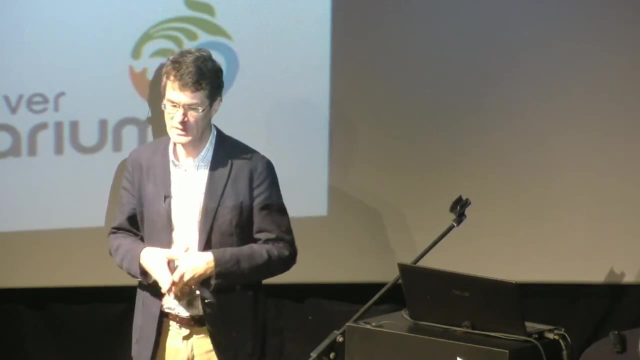 for a very long period of time. It's been used for a very long period of time And they were an oil that was in the form of a transformer oil, industrial grade oil that was used as a either in hydraulic fluids or as a transformer oil. 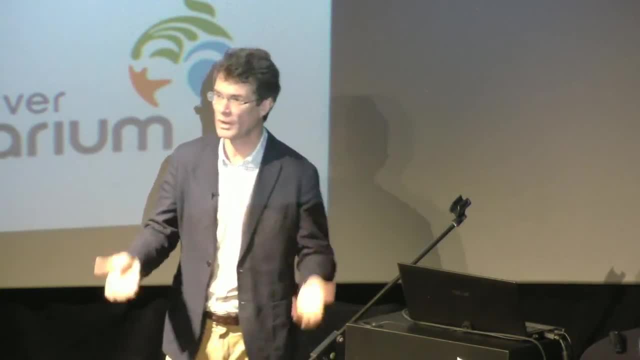 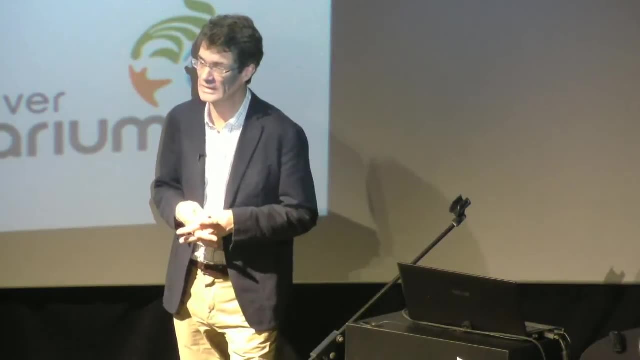 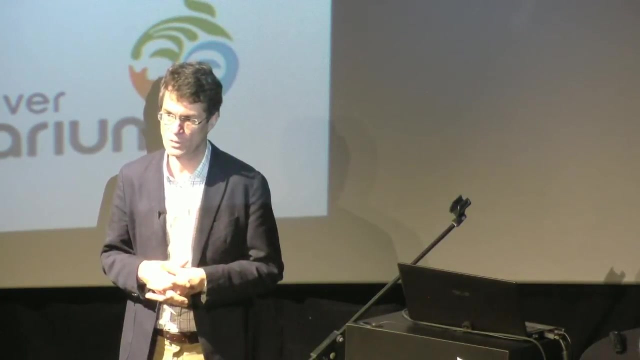 And the reason they were such such a beautiful product from a commercial perspective is that they could transform electricity or lubricate a heavy machine without breaking down, without warming up, without catching fire. And you think, if you think about the history, to become fashionable in the early part of the 20th century, a lot of our structures were made. 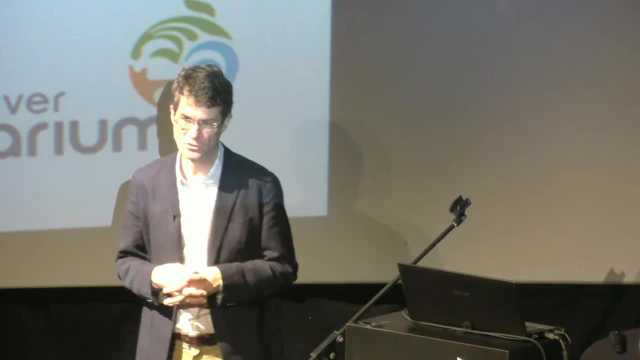 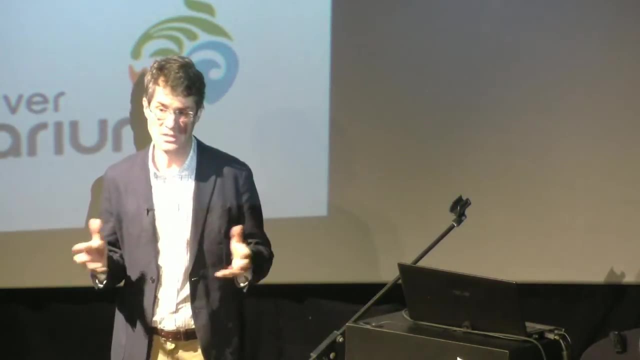 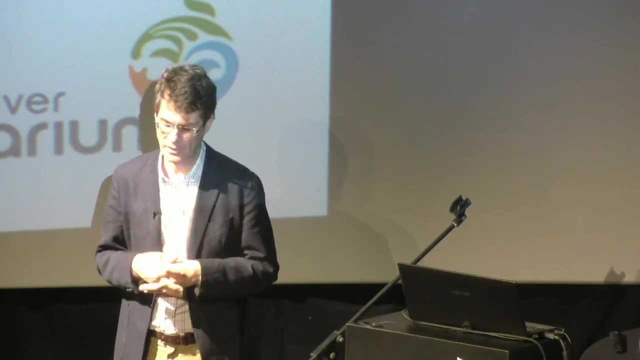 out of wood. so there were tremendous fires when electricity started to ramp up in in our urban areas, and so pcbs were a way to mitigate, if you will, the risk associated with with fire or of fire. and in the same thing, with the radar stations, you have heavy machinery requiring a lot of 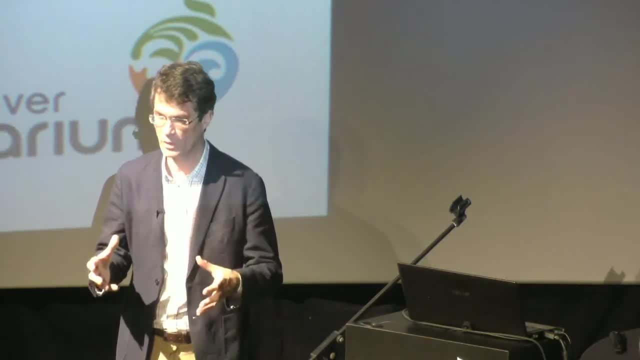 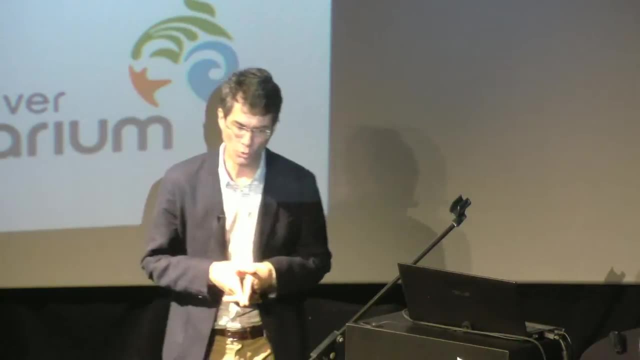 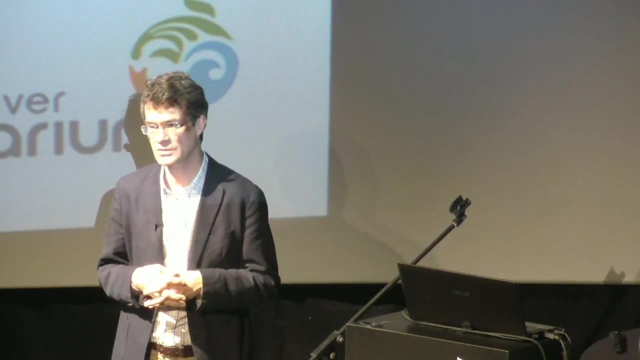 electricity there's a risk of fire. you want an oil that's not going to break down, that's not going to catch fire. pcbs were were great of note today is that mineral oils are used extensively for transformer, as a transformer oil or as a lubricant. so mineral oils are often used by the. 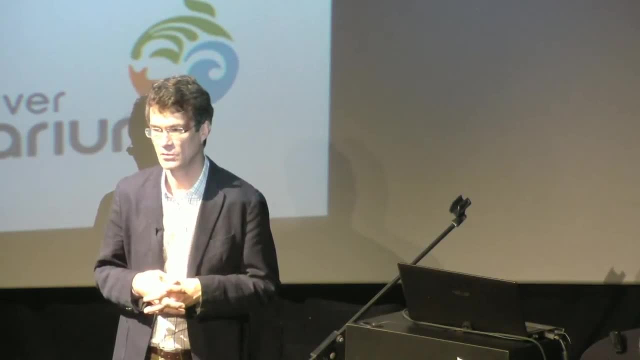 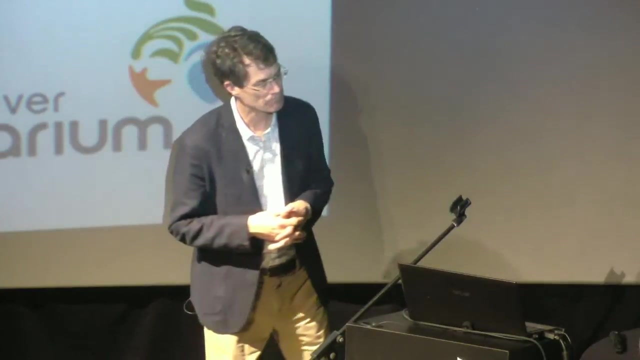 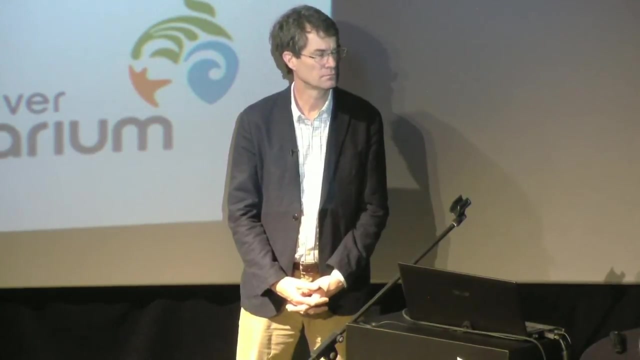 the electric, electricity companies to, to you know, go from the the very high voltage to the household voltage safely, with minimal risk of fire. so okay, so i'm going to read a question here from paula through our youtube channel: have you studied the seabirds that feed or breed in the same area of the seals? have you noticed something in the 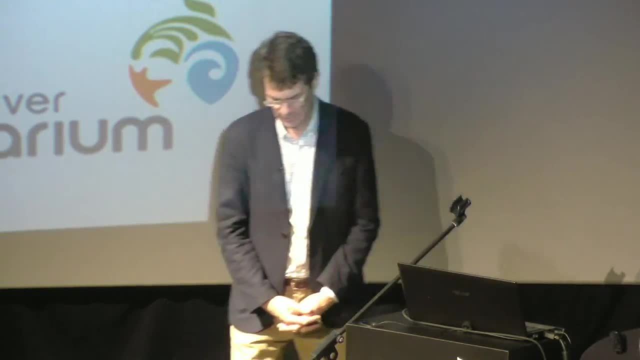 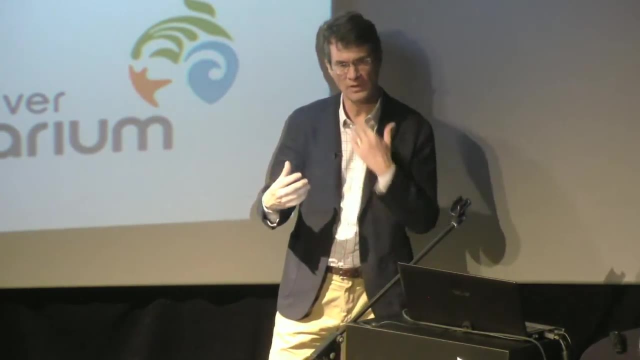 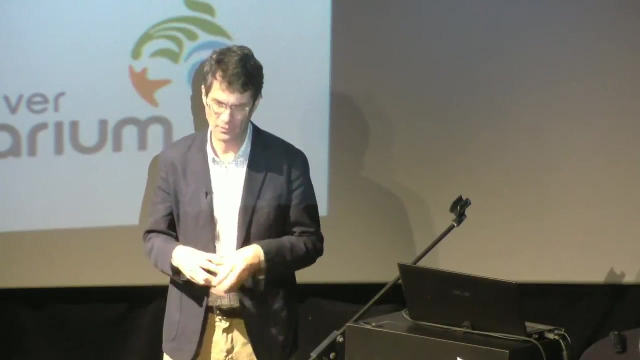 eggshell. so the question uh has to do with seabirds. the pigeon guillemets were the only species of seabird that were studied there. of course, seabirds- if you think about aquatic birds or colonial water birds- often these are ones that eat fish or invertebrates- they're, they're connected. 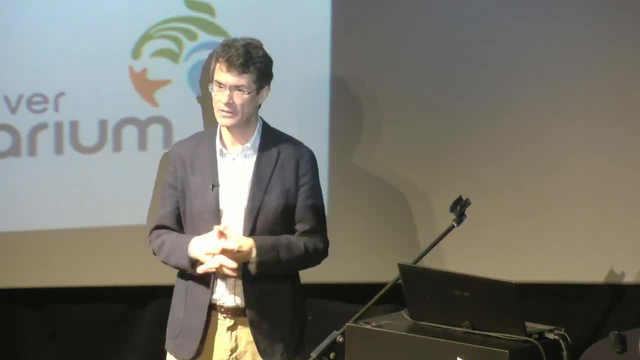 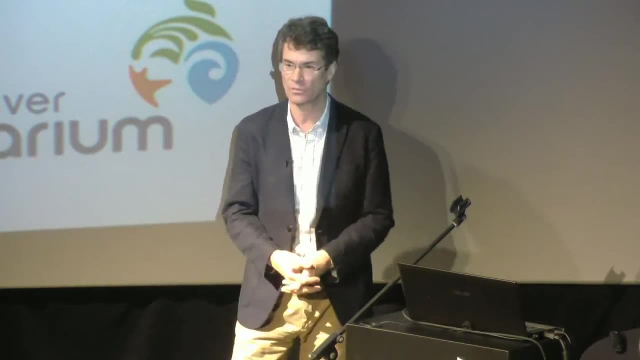 to that aquatic food web. they're not, uh, they're not species that are looking for grains or hanging around you know, crop lands, etc. they're getting down into the water column, they're diving down, they're swimming around, they're, they're picking up fish and in this case, the pitching guillemets. 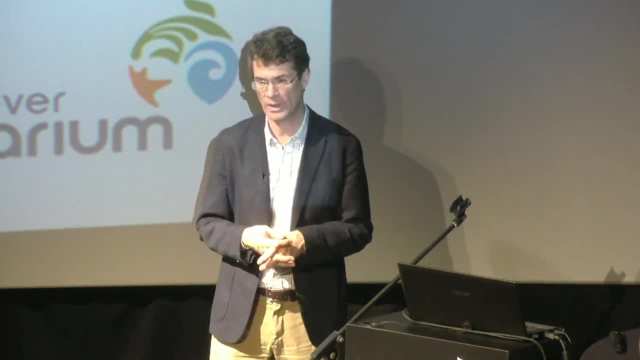 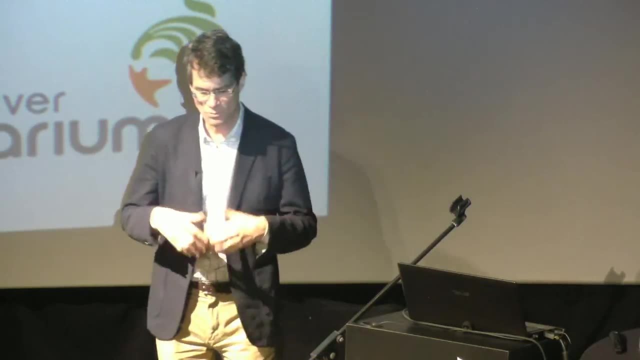 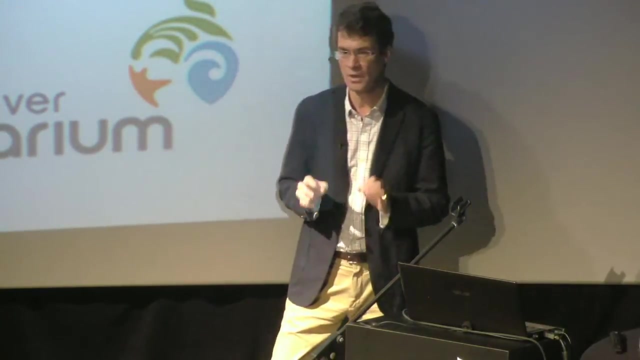 did pick up pcbs from that contaminated food web and that did affect their health. some of the results that i didn't point to here today in terms of eggshell. i would suspect that this the person asking these questions is wondering about eggshell thinning. eggshell thinning was not related to pcbs in the past, but it was related to. 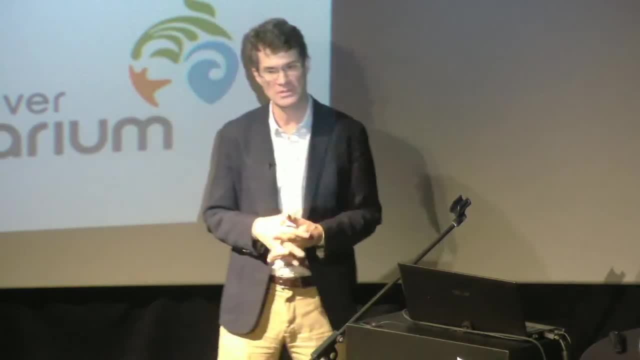 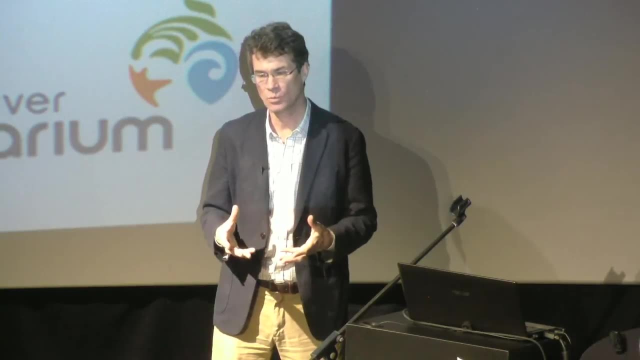 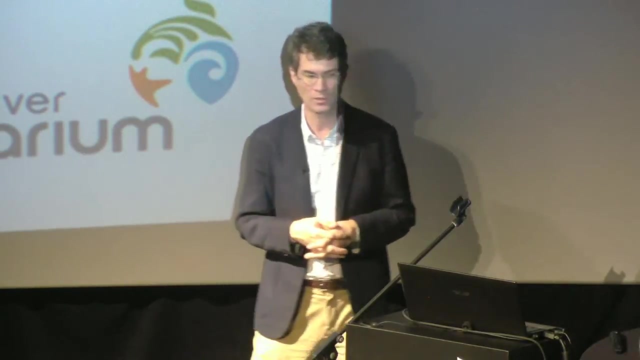 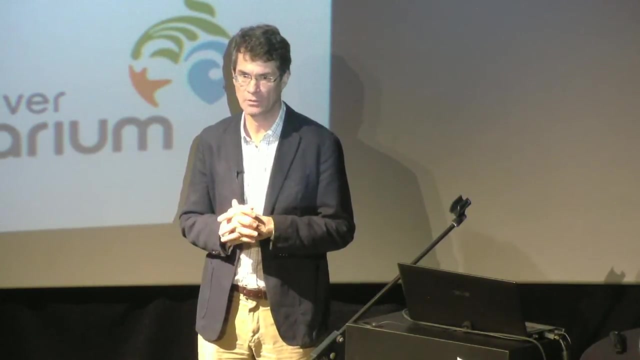 ddt contamination. ddt, the organic chlorine pesticide, also banned about the same era as the pcbs a year or two later. ddt was an organic chlorine pesticide. it was a persistent organic pollutant, so it is one of the stockholm convention. uh pops or pops, and that was a chemical that very uh clearly was resembled estrogen, so it disrupted. 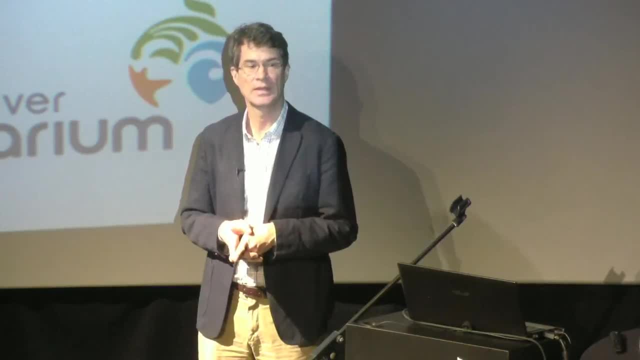 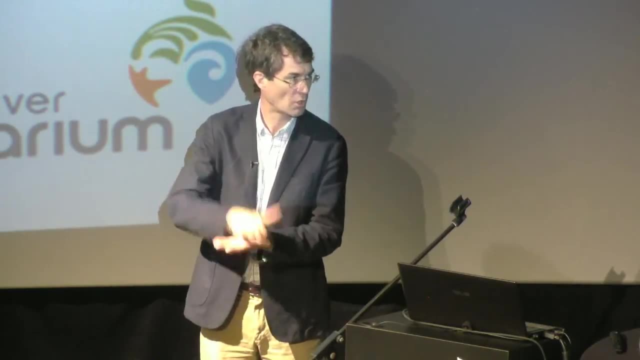 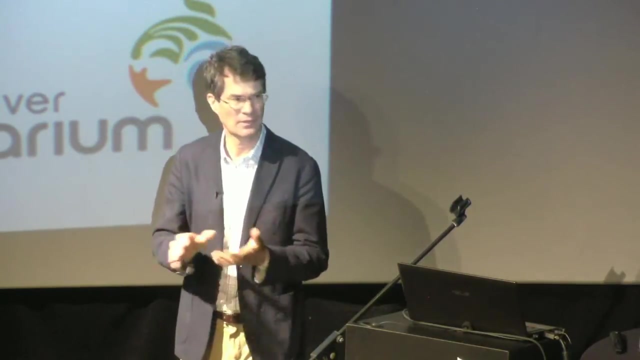 estrogen dynamics in female seabirds and we saw eggshell thinning because of that disruption and the when the females were roosting they would actually crush their chicks and their embryos before they hatched. when the eggshell got to be, i think it was around 14 percent thinner than 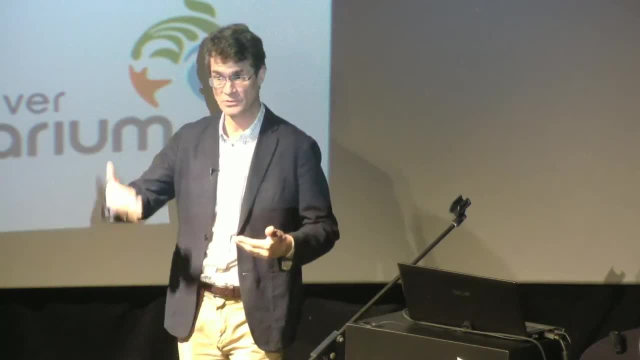 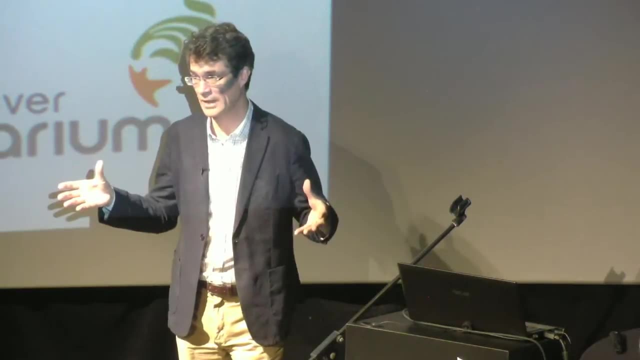 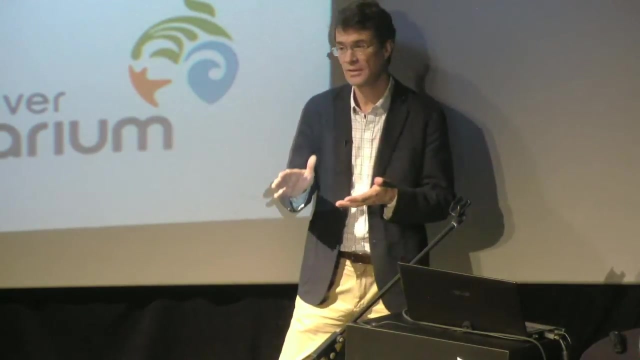 the eggshell. so ddt caused a disruption in calcium dynamics because of a disruption in estrogen physiology led to a thinning of the eggshell and we saw widespread extirpation, ie localized uh extinction of a lot of seabirds, double crested cormorants in the great lakes, bald eagles, peregrine. 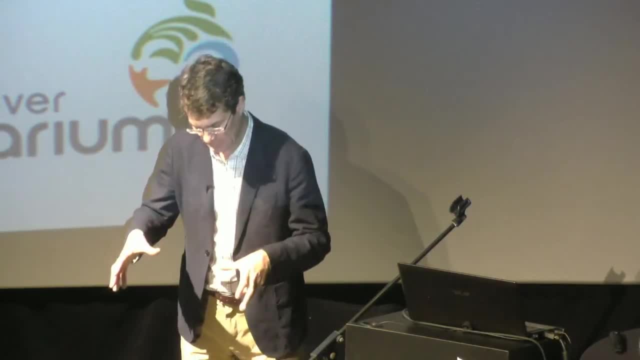 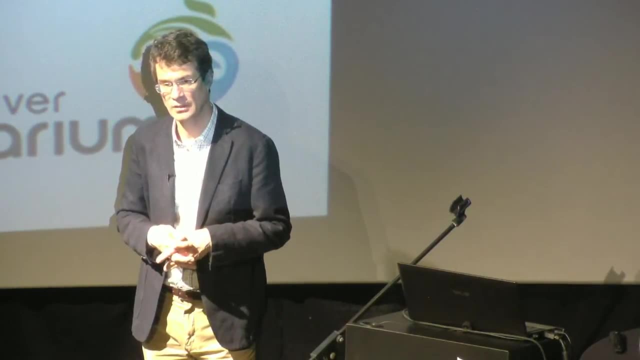 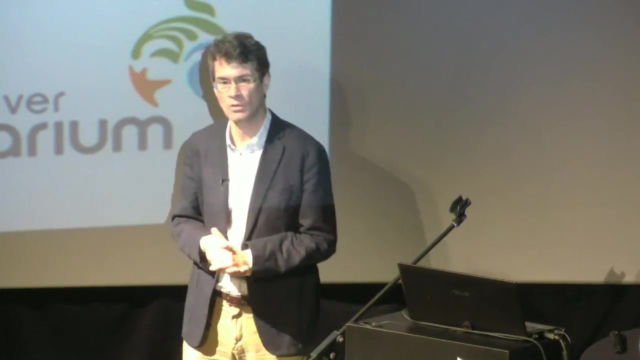 falcons, pelicans, a lot of different species of birds that were relying heavily on aquatic food webs, were getting exposed, affected by getting in, taking in too much DDT, across the continent of North America and Europe and Asia. so, eggshell thinning. another interesting story, probably the preeminent story of wildlife toxicology, if you're looking. 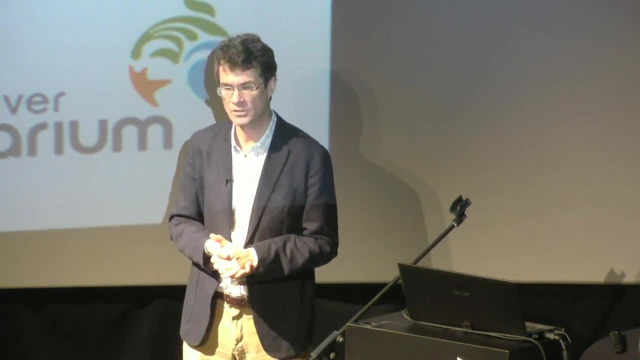 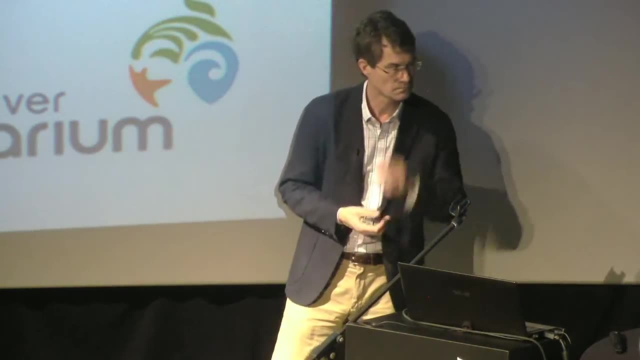 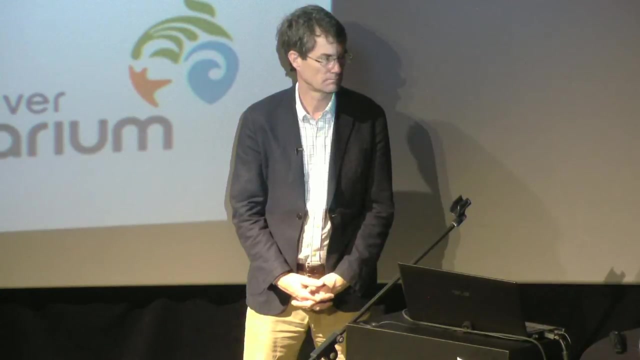 for population level. consequences of impact associated with a single chemical. it's DDT, and it was a nasty story, all right. and our next question is from Zach, also through our YouTube channel: how many PCBs does it take to contaminate wildlife? how many PCBs does it take to contaminate wildlife? well, the 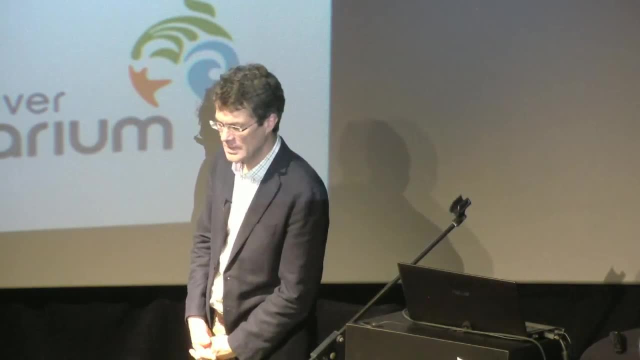 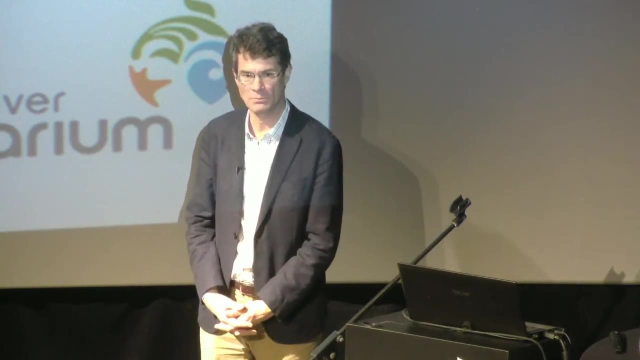 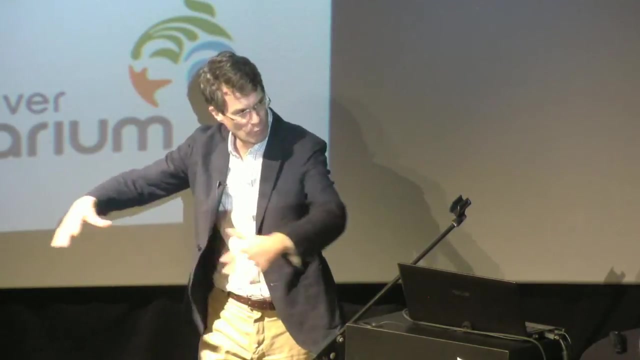 interesting thing. that's a very difficult question to answer, but it doesn't take a lot. if we look at sag like Bay, for example, is 450 kilograms of a very, very thick oil, most of which stayed very close to the contaminated site. you saw that red zone where that thick oil stayed and it took two weeks to get rid of that thick oil and it took about a week to get rid of that thick oil. and it took about a week to get rid of that thick oil and it took quite a lot of a long time for that. that thick oil to sort of weather and 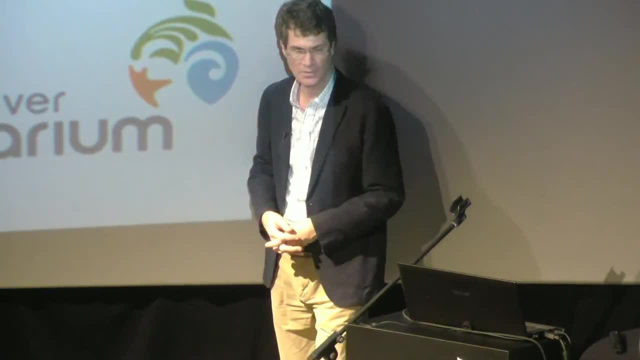 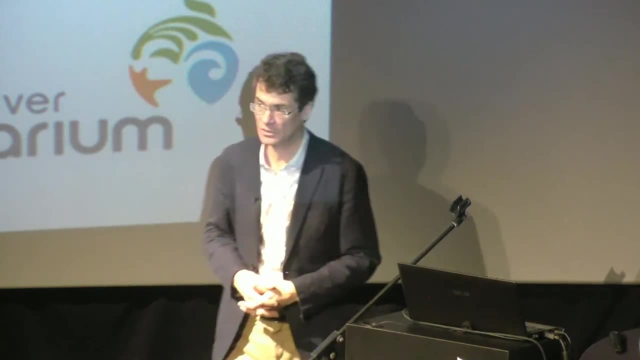 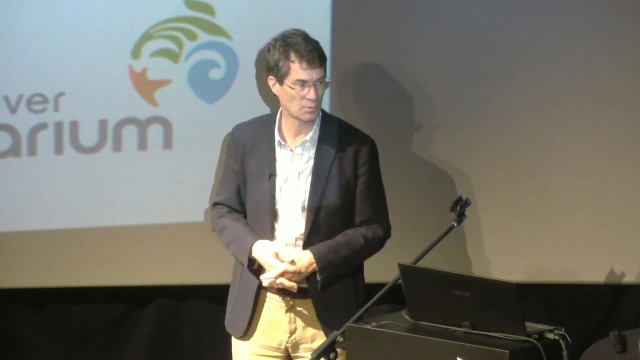 move out away from that source. so PCBs tend not to move very far. but it doesn't take a lot. you saw that single spill led to contamination of the entire food web within that that fjord, well beyond the boundaries of the of the contaminated sediments. it does not take a lot. yeah, I think I would leave it there, all right. 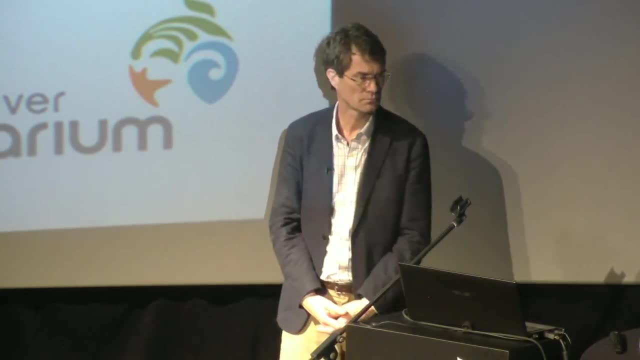 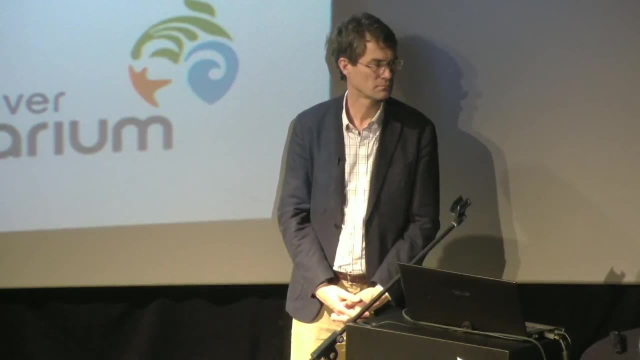 great, we do have a third question, the. the question is about: can you talk a bit about the cetaceans? and I'm gonna, I'm gonna make the assumption that maybe in in the context of contaminants, because we've been talking a fair bit about those, next we have some other classes or we'll talk a fair bit about the natural. 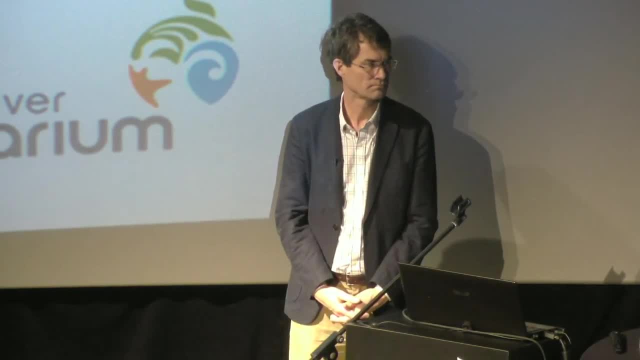 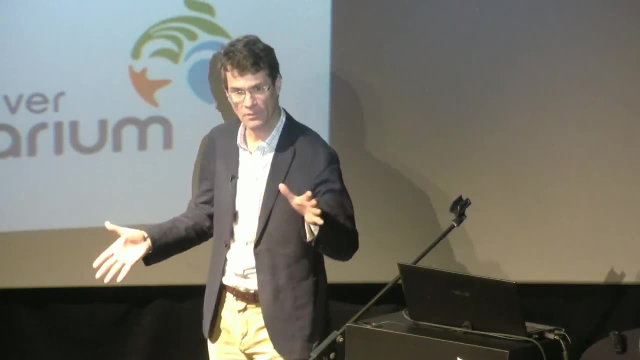 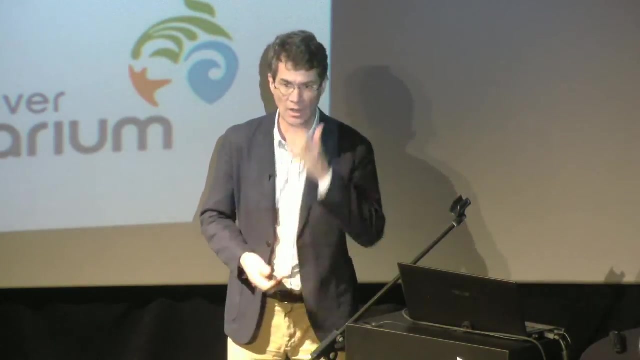 history of cetaceans. so do you want to make any comments on cetacean contaminants? sure, I mean, cetaceans are marine mammals, but within all the marine mammals that we, that we know from all over the world, there are a number of different life histories. we've got very long lived. species- bowhead whales- we now think to live or long time. we've got the ring seals that live maybe 35 or four years, forty years. we've got the killer whales off our coast here, where females can live to be 80 or 90 years- a long, long time. so some of these species were, and some of the species that depend on my anteaters don't have over 500 thousand to have a huntees, so some of these species that can livecią long time are 80 or 90 years. 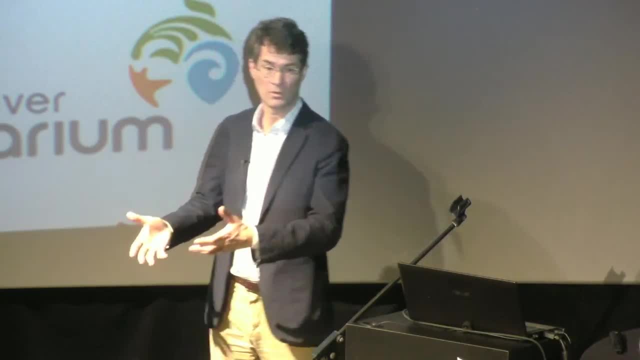 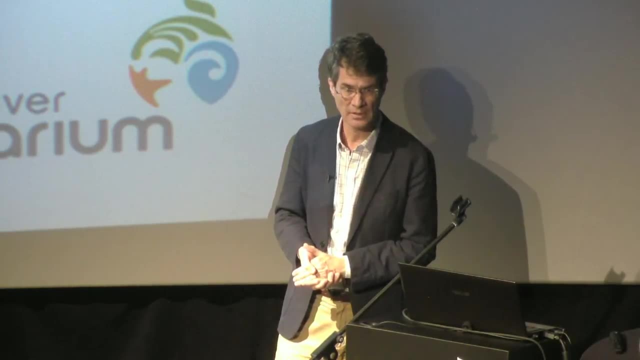 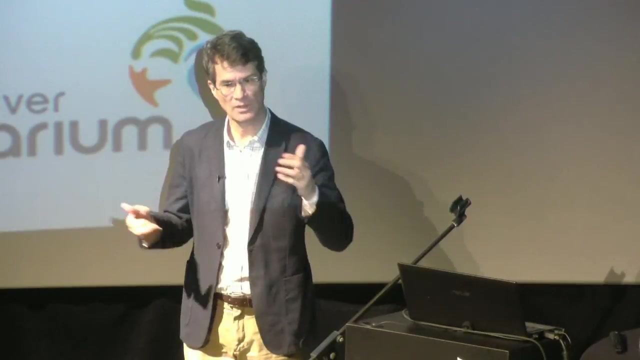 A long long time. So some of these species and some of the individuals within these populations were born before PCBs or DDT were invented commercially. So we've seen they have borne witness to a lot of big, big changes. If we look at the whales, we've got different types of whales. 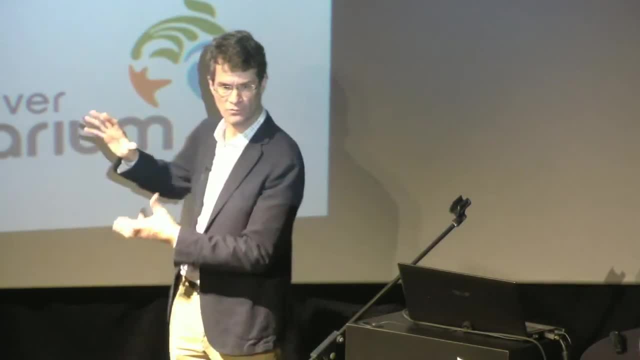 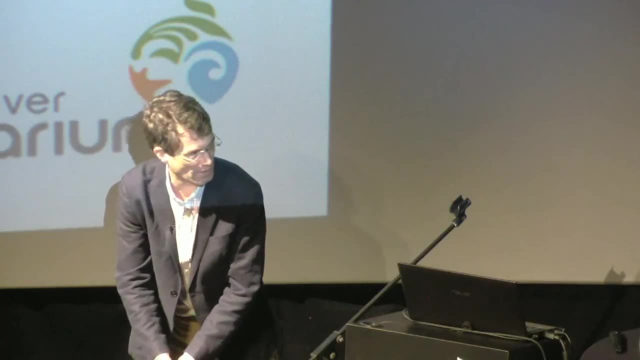 So when we're looking at contaminants, just think back to that food web. What does the food web look like? Are we talking a gray whale which dives to the sediments and takes a mouthful of mud and pushes its tongue out and filters out all of the different invertebrates? 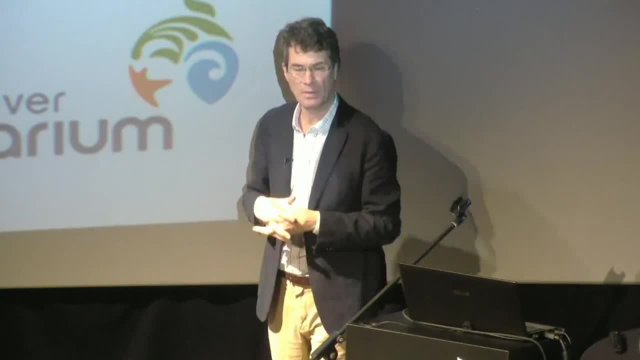 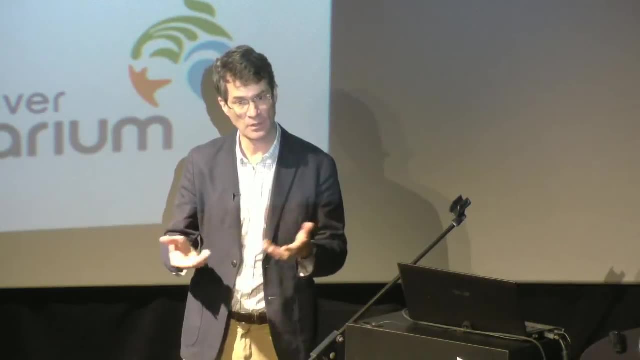 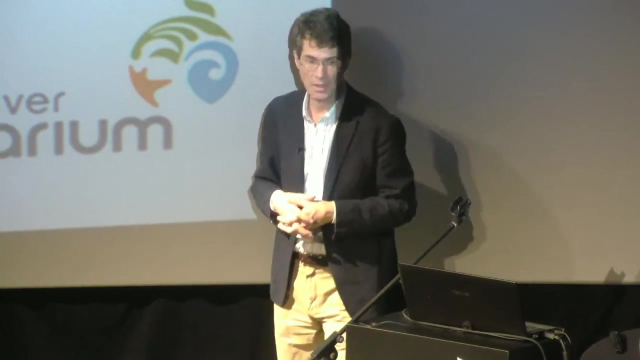 and swallows and retains those. Are we talking about humpback whales that might bubble, feed and capture herring, a school of herring, and feed on those fish, those smallish fish in the water column? Or we think about killer whales, transit killer whales? 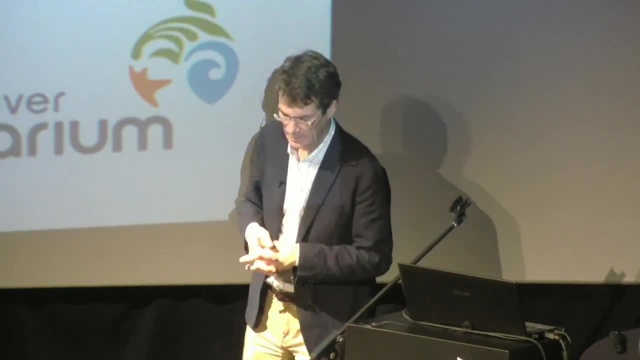 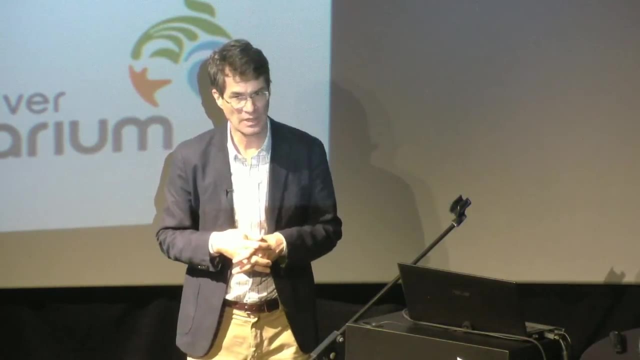 or bigs killer whales, as the transit killer whales here are called, that explode. So we've got a lot of different types of marine mammals. So if we have similar ecotypes in the Northwest Atlantic- and we do- and they're feeding on marine mammals, 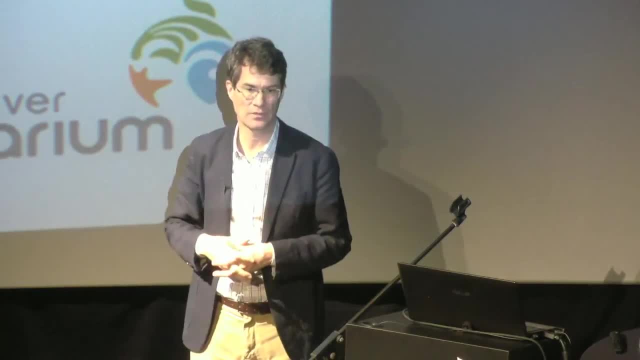 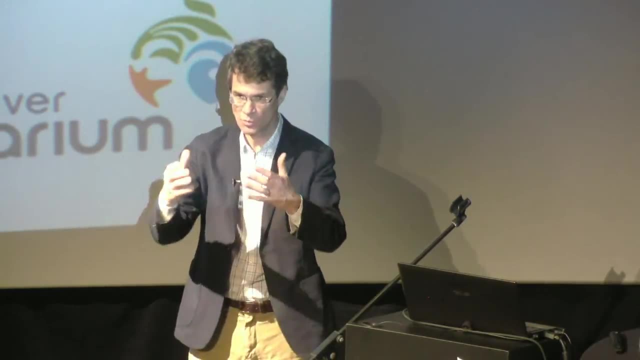 then they're one step higher in the food chain than the ring-sealed that's already contaminated. So when we look at the persistent organic pollutants or the PBT chemicals- those with persistence, those with biocumulative tendencies and those that are toxic- 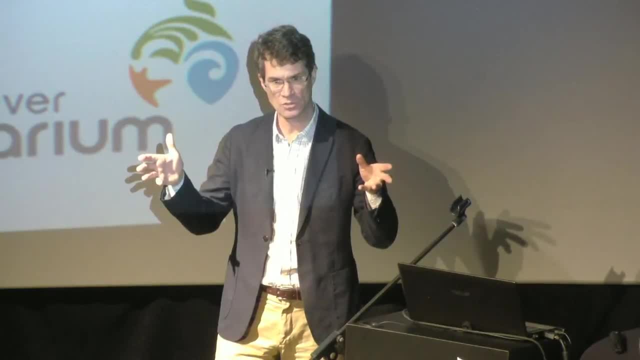 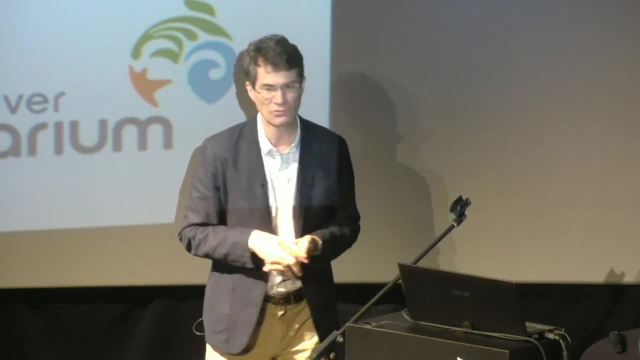 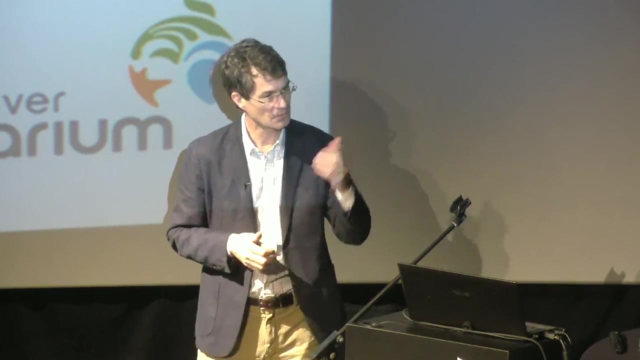 we worry most about long-lived creatures at the top of the food chain. That's where we see the highest degree of contamination And that's why we worry about some of these endangered whales, certainly the killer whales around here and some other species that we'll hear about in another course. 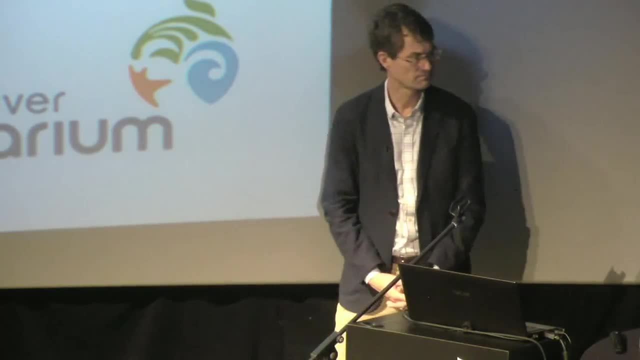 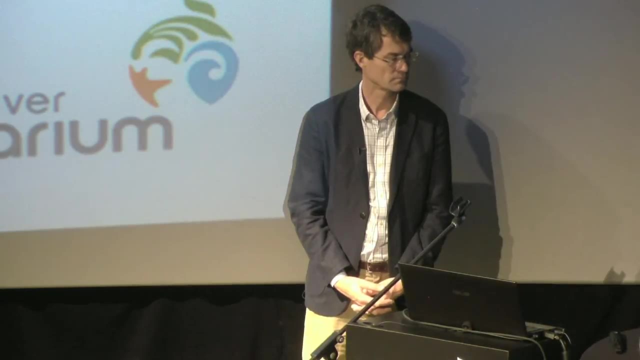 All right, great. Thank you, Nathan. had a follow-up question but, Nathan, I'm going to ask for your patience because we're going to talk a bit more about cetaceans in some other classes, So I want you to tune in for those and bring your questions back for those. 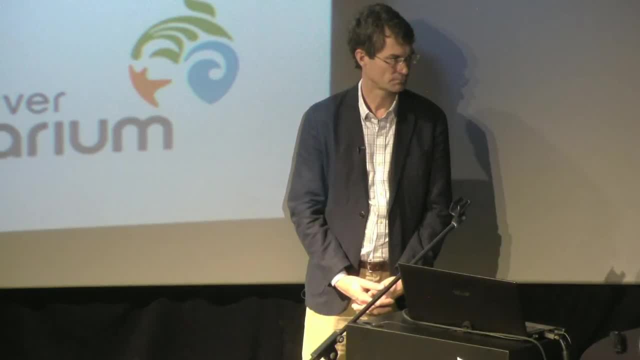 And a final question. A final question for Dr Peter Ross tonight: Is the melting of the ice affecting the sedimentary process of layering on top of the PCBs? You talked a bit about that layering. That's an excellent question. 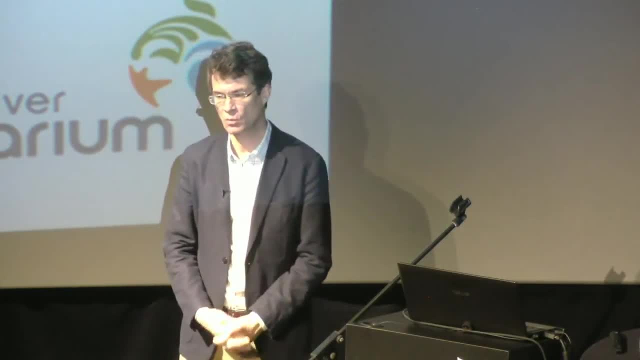 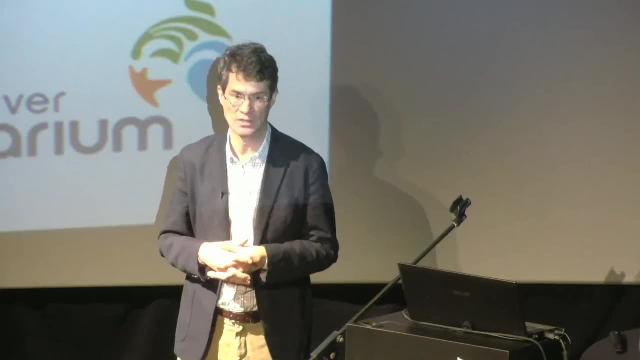 And, of course, the Arctic is changing as we speak, and it's changing quickly. We do worry about what that means, both in terms of, you know, the biology and ecology. A lot of these ice-associated species, whether it's ring-seals or caribou, that have to transit. 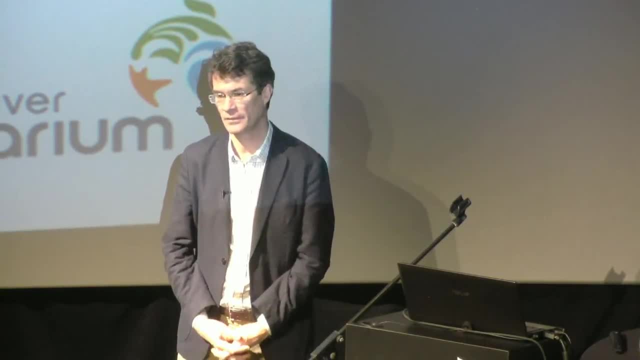 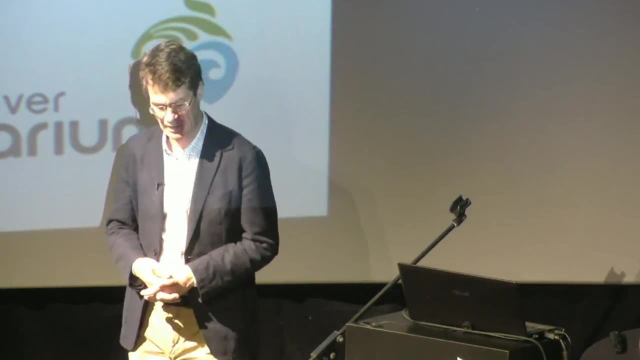 from island to island, or polar bears that are looking to feed off ring-seals. So climate change is very real in the Arctic and presents a very grave danger to a way of life of many different species, as well as the Inuit that rely on these. 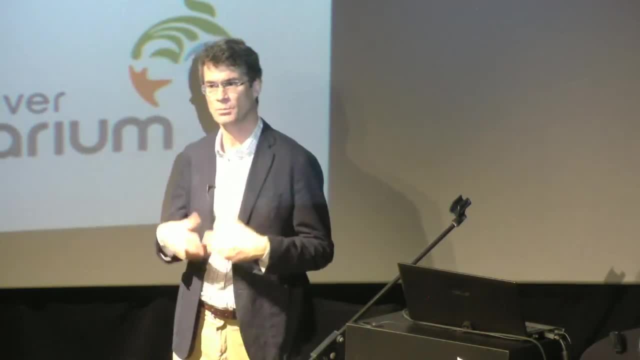 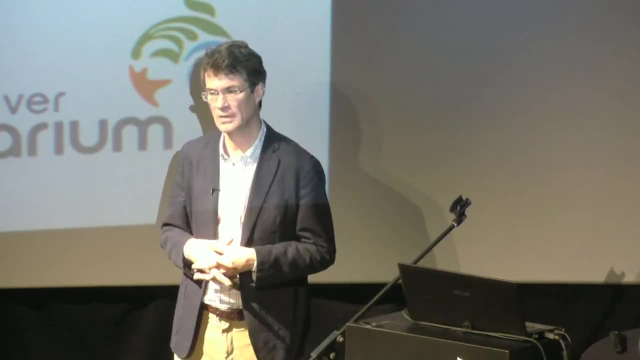 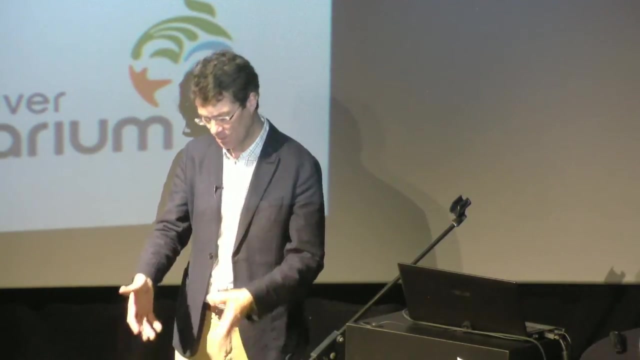 In terms of pollution, though. climate change has the potential to greatly alter the way in which different types of pollutants move around the environment. If you think about pollutants that are traveling through our air- so air pollution- they may be dropped out onto a river. Into a body of snow or ice and then that's where they lie until springtime, and then they might evaporate, They might get into the water column. If that ice disappears, those pollutants are going to enter the water more quickly and 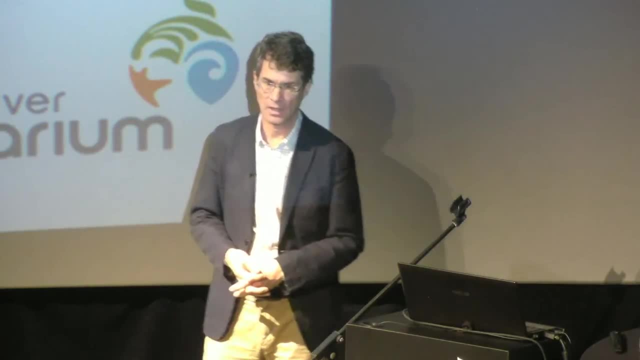 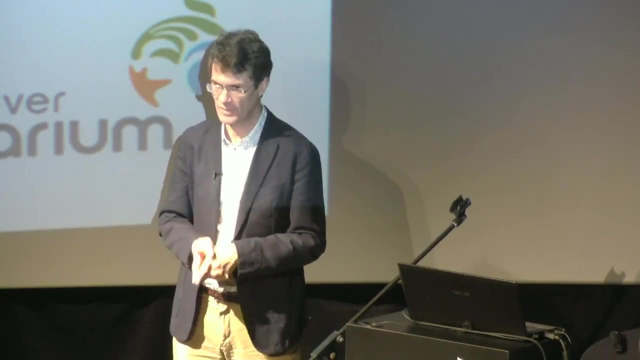 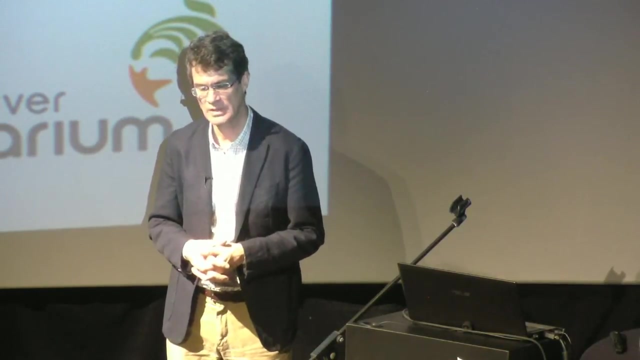 other pollutants might evaporate in a different manner. So climate change is going to change a lot of the functions related to transport and fate of different types of contaminants, and that's something we are watching for In the Arctic, no question, In terms of sedimentation and some of the other processes, absolutely.